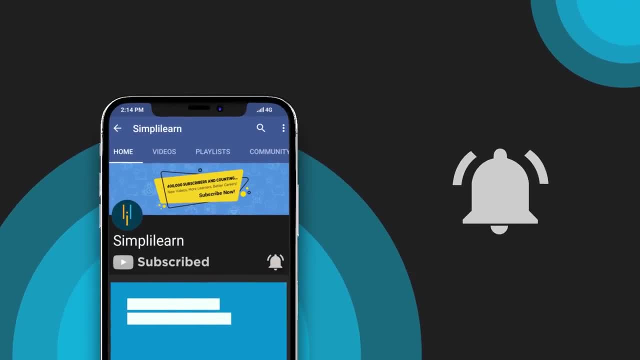 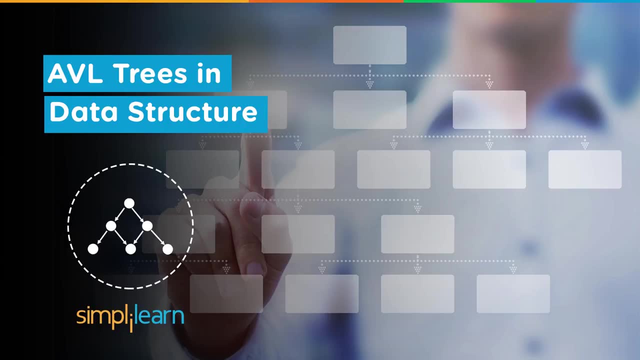 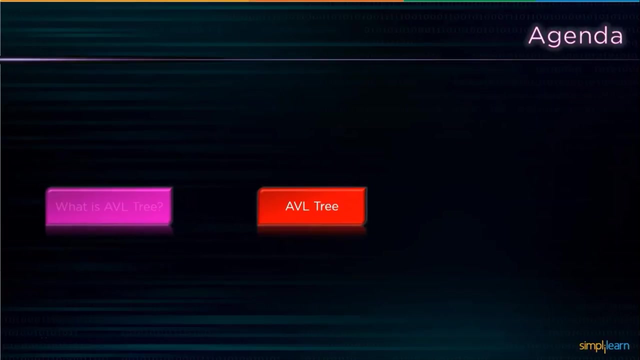 Hey everyone, I am Babak Handelwal and I welcome you all to Simply Learn's YouTube channel. In this session we will talk about avial trees. We shall begin our session by what is an avial tree, Then we will discuss various rotations we can perform to balance avial. 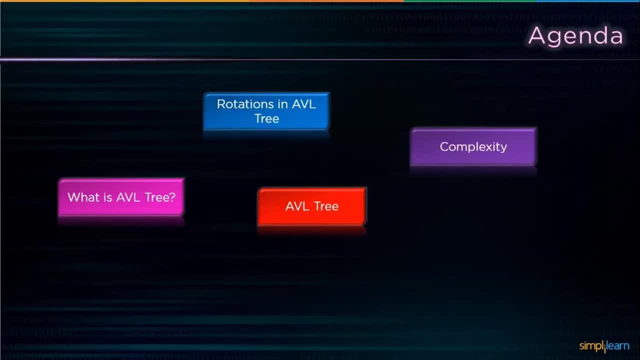 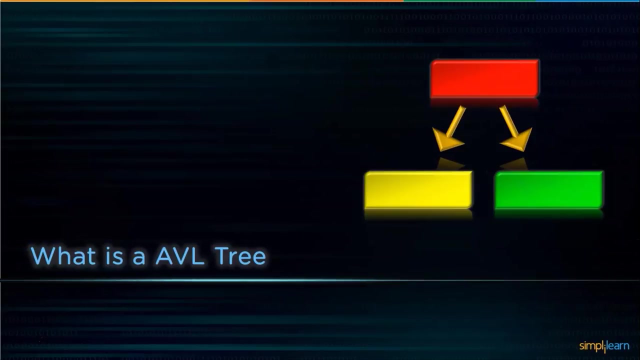 trees. Then we will discuss the complexity of avial trees. After that we will try various operations on them, like insertion, deletion. Finally, we will sum up what we have learned from this session, But before we begin, make sure you have subscribed to our YouTube channel. 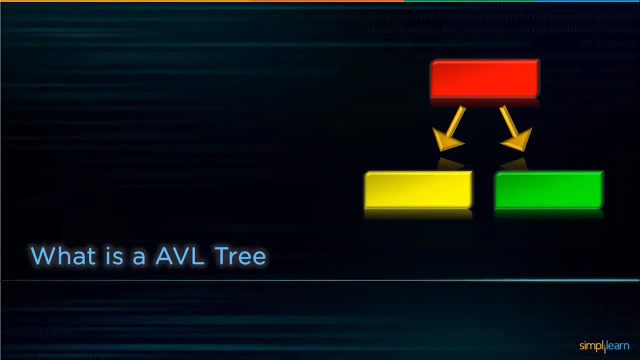 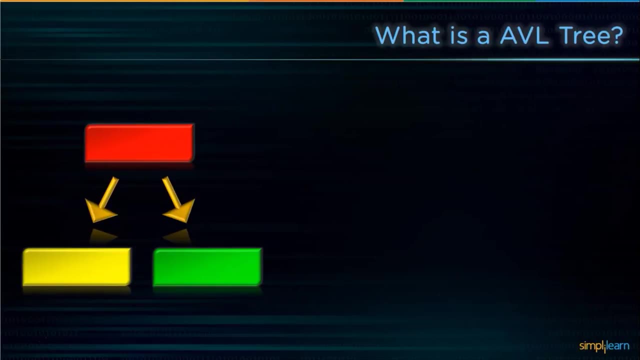 and clicked on the bell icon below so you never miss an update from Simply Learn's YouTube channel. So let's get started with introduction to avial trees. An avial tree is a height-balanced pine tree. An avial tree is a height-balanced pine tree. 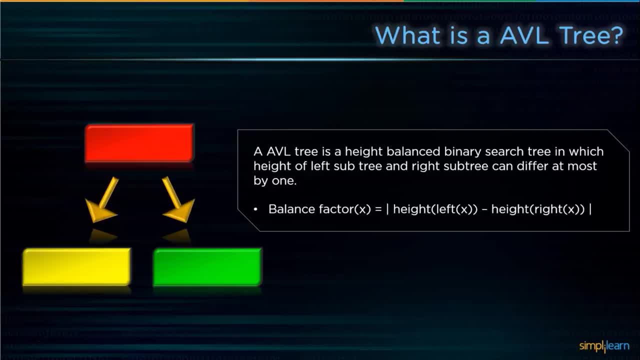 is a height-balanced pine tree. For each node, we have to make sure that the height of the left subtree and the right subtree can differ by at most one. We can calculate this balance factor by subtracting the height of the left subtree from the height of the. 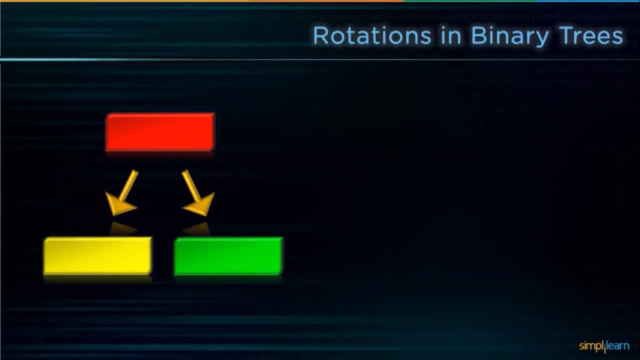 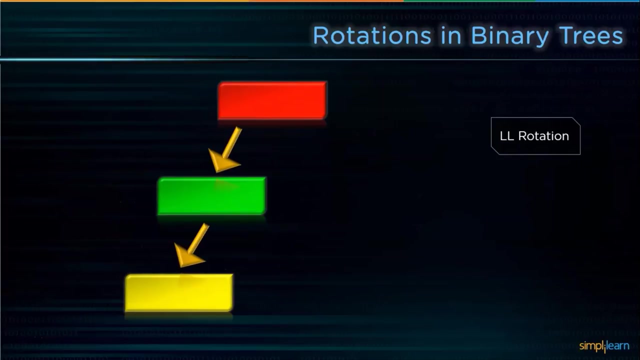 right subtree. Now let's discuss various rotations we can perform on avial trees. First up, LL rotation, Next RR rotations, Next LR rotation, At last RL rotation. Let's discuss them in detail. First up, LL rotation. It is a clockwise rotation. When a node is 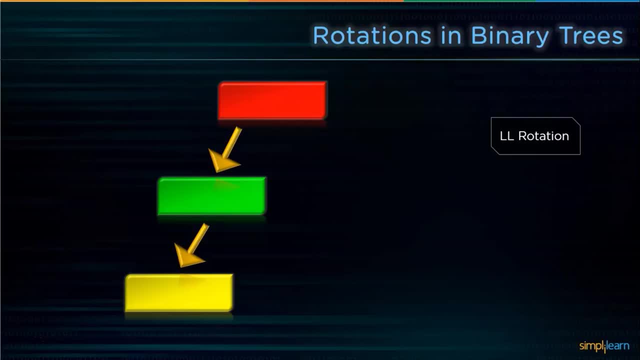 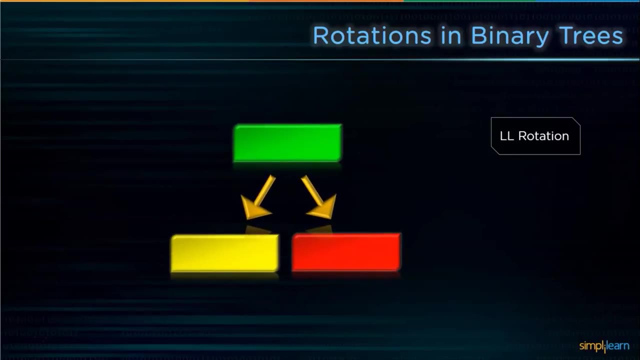 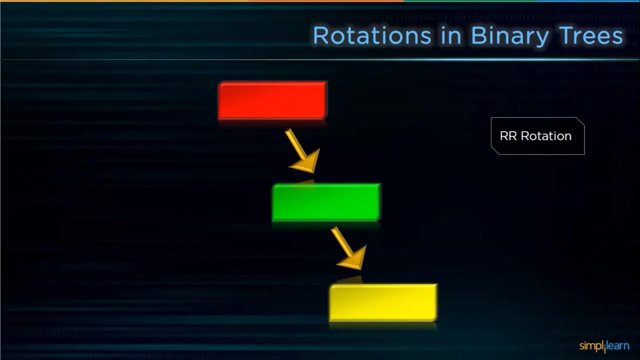 inserted on the left subtree of the left subtree of a node, then we apply this rotation to balance the tree. It is applied on a node below the balance factor 2 node, That is, we will apply right rotation on the green node, Next RR rotation When a node is inserted. 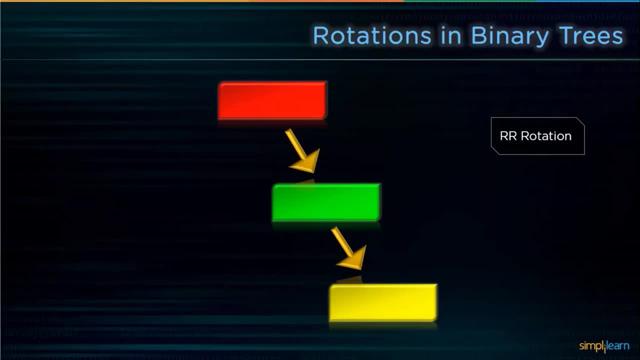 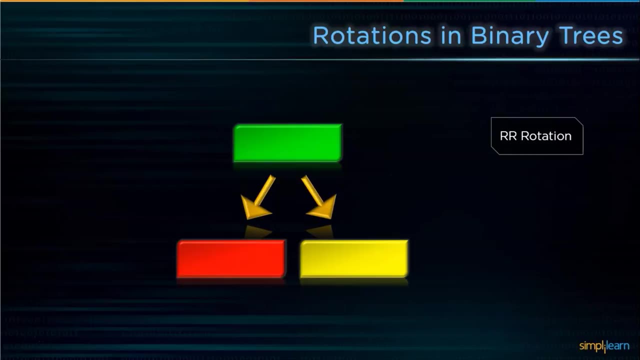 into a right subtree of the right subtree of a node, then we perform RR rotation. It is an anticlockwise rotation When a node is inserted into a right subtree of the right subtree, rotation which is applied on the node below a node having balance factor minus 2, that is, we will. 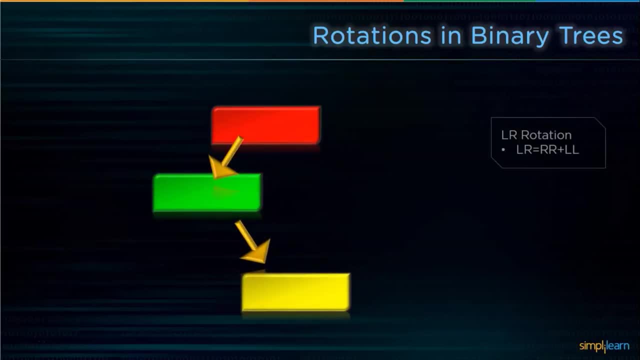 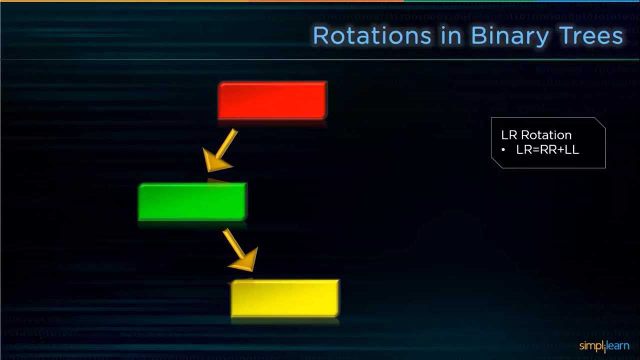 apply it on the green node. Next up LR rotation. When a node is inserted into right subtree of the left subtree of a node, then we perform LR's rotation. It is a combination of RR and LL rotation. First we will apply RR rotation on green and yellow node, After this red. 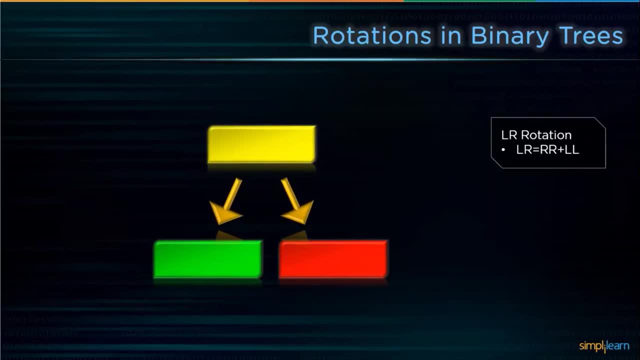 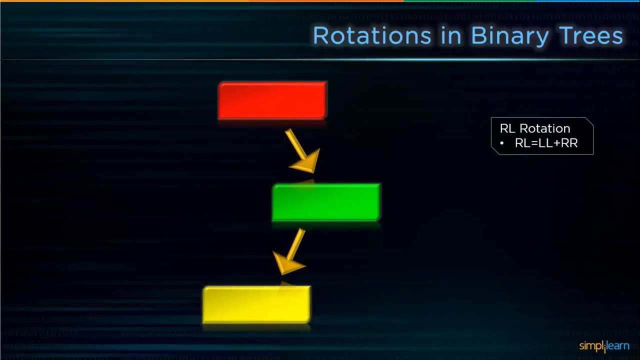 node is still unbalanced, so we will perform LL rotation on the yellow node. Finally, RL rotation: When a node is inserted into the left subtree of right subtree of a node, then we perform RL rotation. It is a combination of LL and RR rotation. First we will apply LL rotation on green and yellow nodes. 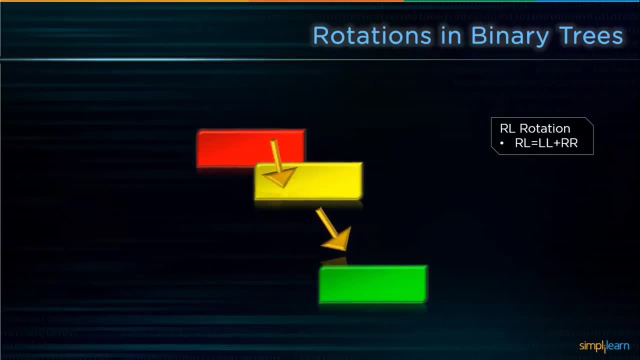 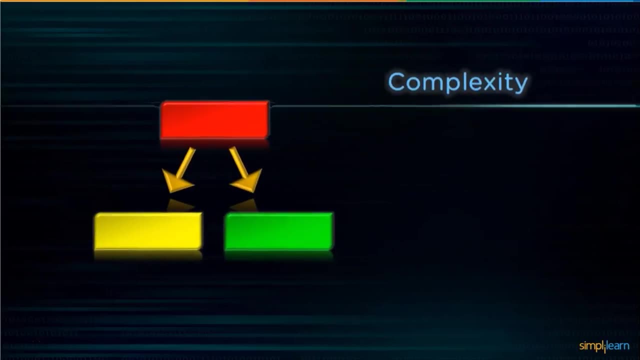 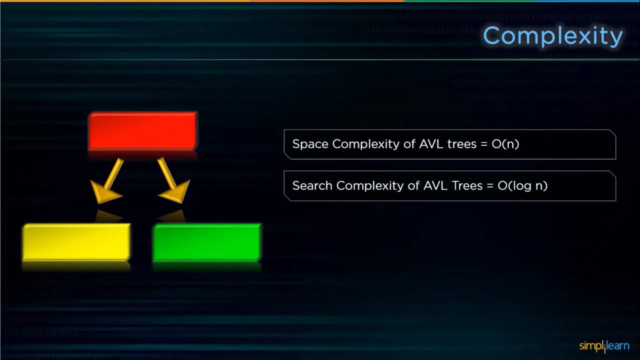 After this, the red node is still unbalanced, so we will perform RR rotation on the yellow node. Now let's discuss complexity of avial trees. First up, space complexity is a bigger of n. Next up avial tree offers a complexity of bigger of log n for searching Next up. 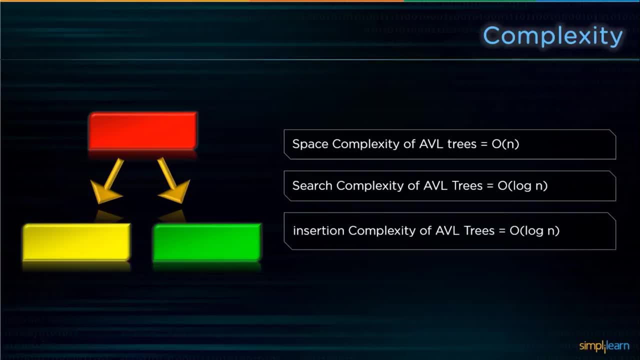 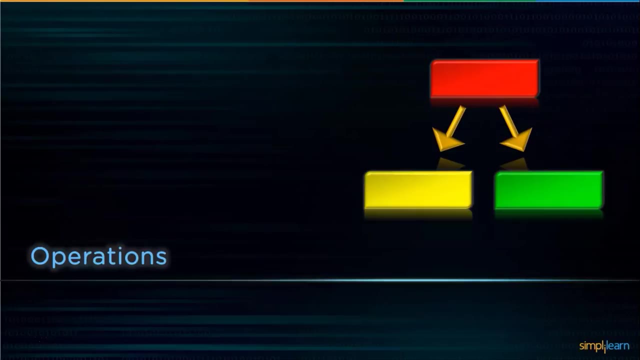 avial trees offer a complexity of bigger of log n for insertion. Finally, avial tree offers a complexity of bigger of log n of for deletion. We have now introduced an avial tree and rotations on it. Now let's discuss some of the operations we can perform on avial trees. 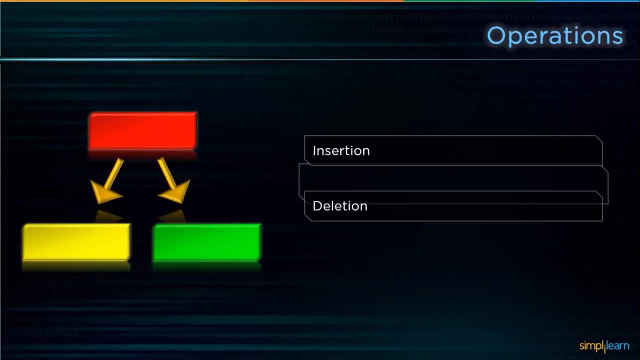 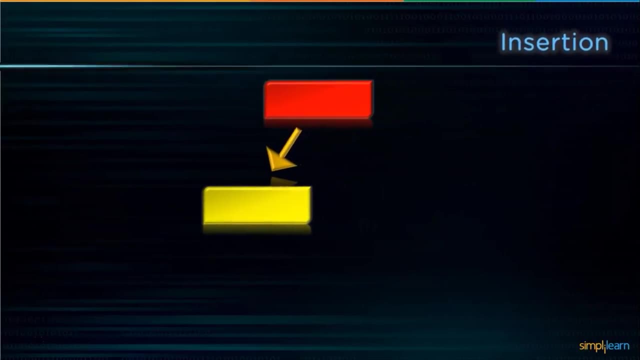 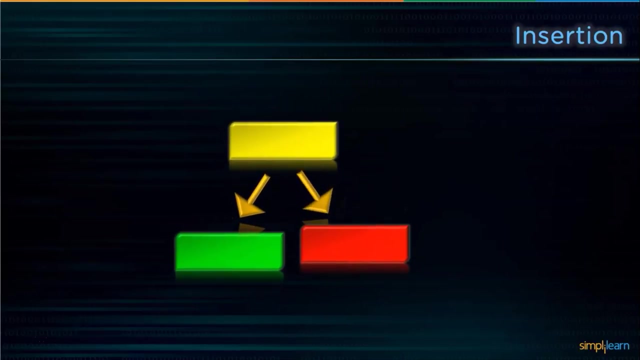 First up: insertion and deletion. Let's discuss them in detail. First up, insertion. We will insert a node following binary search tree rules. Then we will check if the nodes are balanced or not. If they are not, then we will balance it by using suitable rotations. 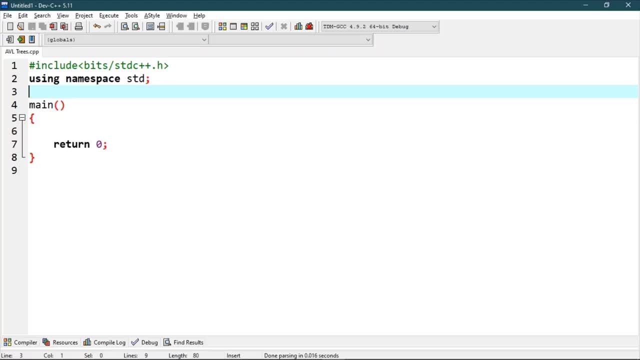 Now let's try these operations. Let's start by creating a node. To create a node, we need a class node. We will create its member as public int key node: star left- dcin2성을node. star right. int height: h pies og up. 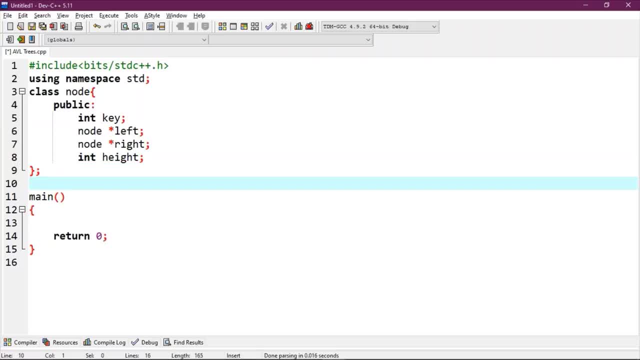 int private. int. int private, out, out out, send, send, check. Let's write a function to get maximum of two integers, So int max, int a, comma, int b. Now let's declare a utility function to get maximum of two integers, So int max, a, comma, int b. 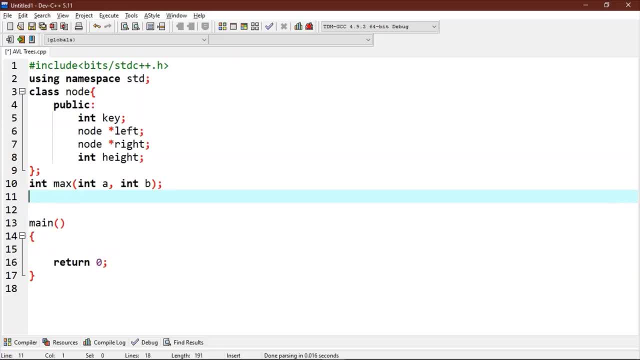 Now let's write a function to get the height of the tree: Int height, Int height: Node star n. Now, if n is null, then we will return 0, else we will return n calls height. Now let's write that function to get maximum of two integers. 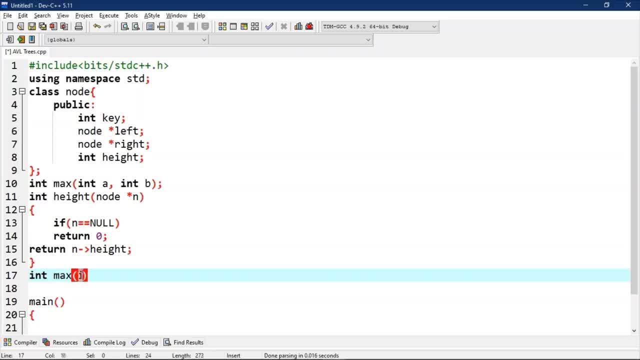 Int max, int a comma, int b. Now let's write a function to get maximum of two integers. So: int max, int a comma, int b. Now let's write a function to get maximum of two integers. Now let's write a function to get maximum of two integers. 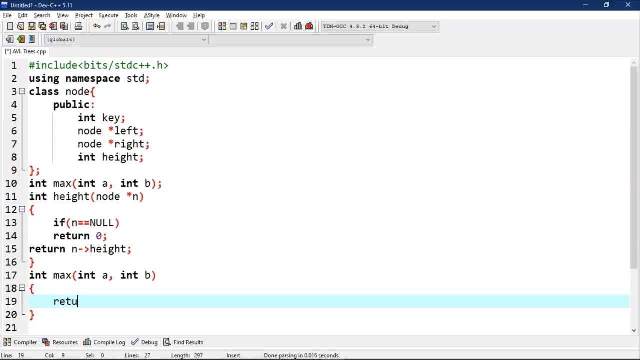 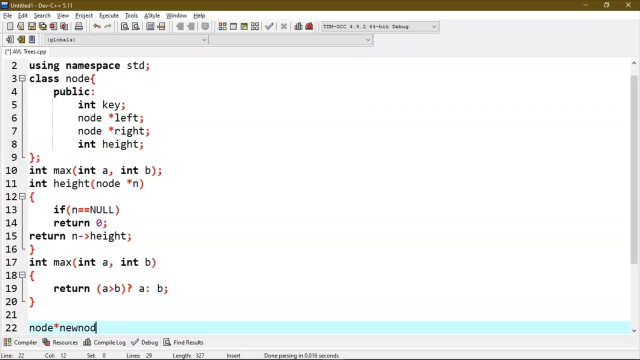 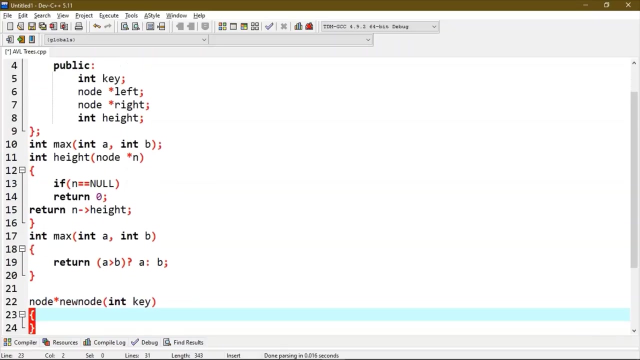 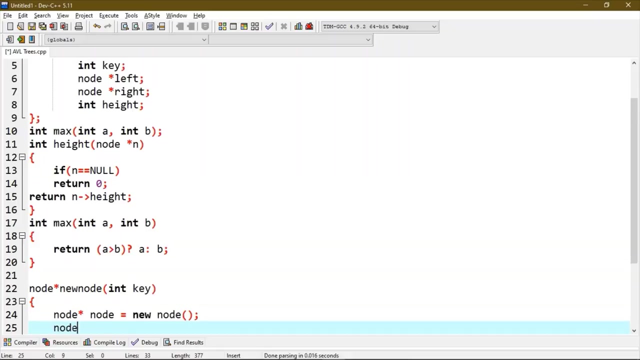 We will return. if a is greater than b, then we will return a, else we will return b. Now let's write a helper function that allocates a new node with a given key and null left and right pointers. node star- new node and key node star node equals to new node, so node. 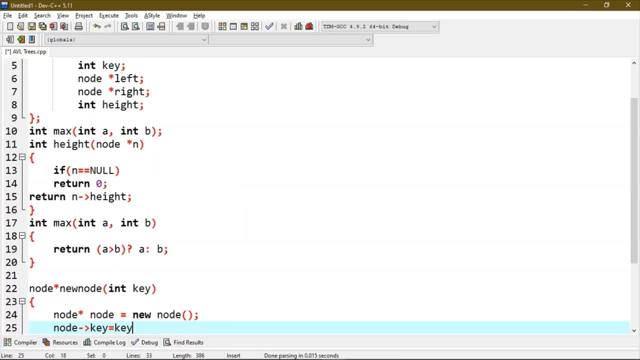 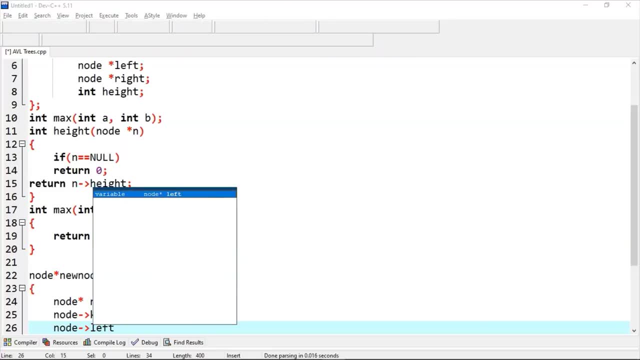 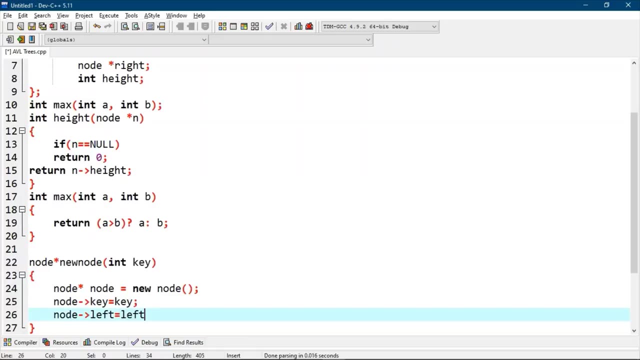 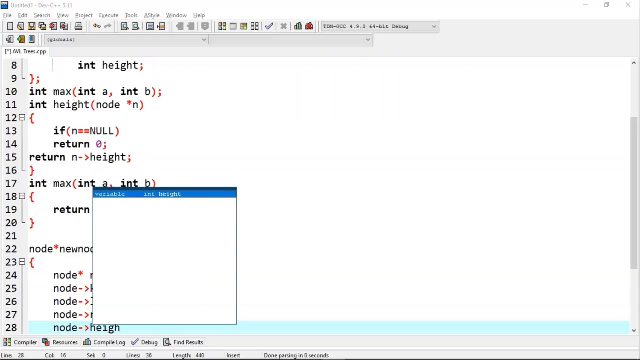 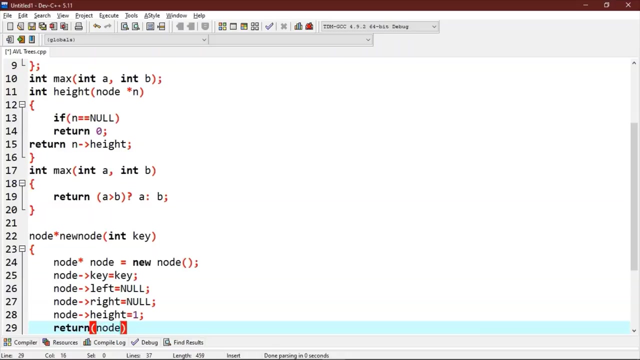 key will be equals to key, node left will be equals to left, node left will be equals to null and node right will be equals to null and node right will be equals to one and return node. Here we have kept height as one because at the new node is initially added at leave. 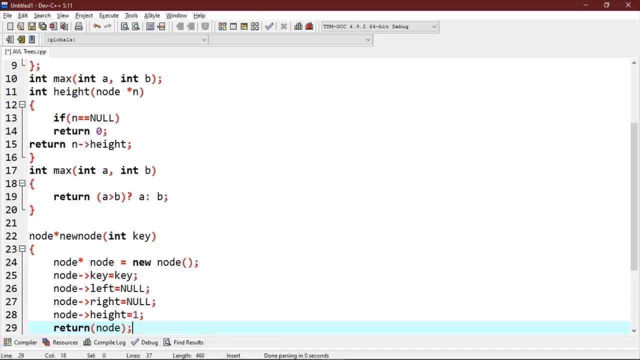 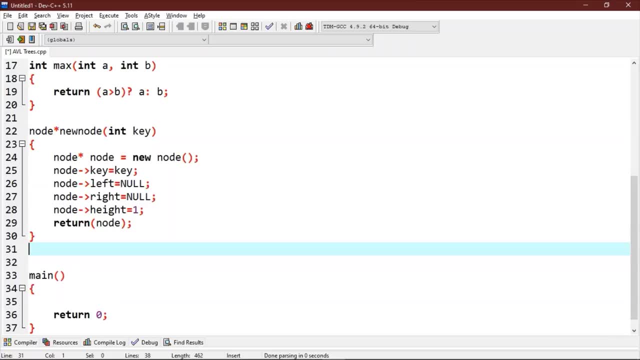 so by default, it will be always be at one. Now let's write a utility function to right rotate subtree rooted with variety. Now Let's write a utility function to right rotate subtree rooted with variety. That's it, Thank you. 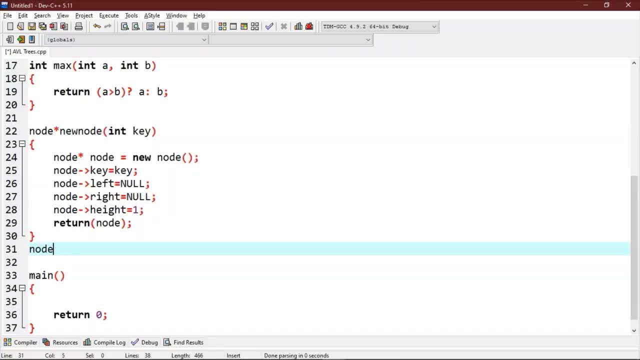 Byee. node star right, node star y, now node star x, is equals to y's left and node star e2 is equals to x. right now we will perform rotation, so x right will become y and y's left will become t2. now we will update the heights. 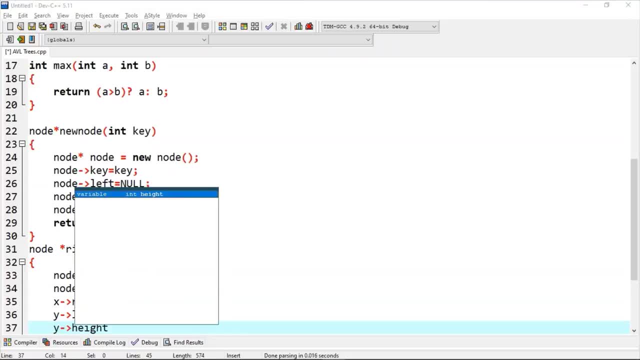 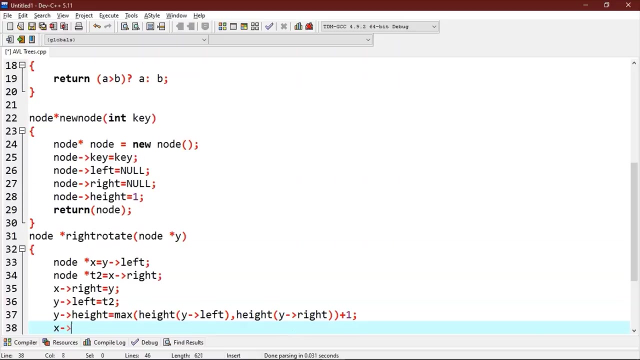 so y height is equals to max of height of y left comma height of y right plus 1 plus 1. now x height equals to maximum of height x left, left comma. height of x right of x right plus 1 plus 1 plus 1. 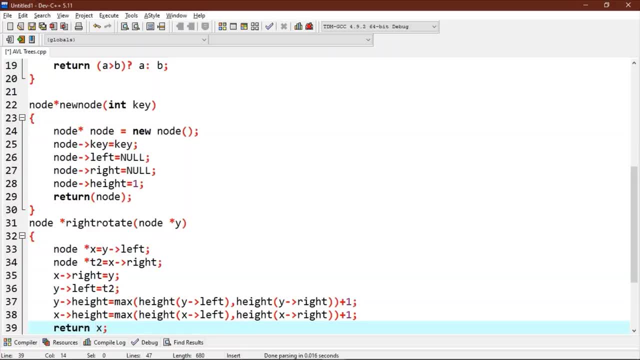 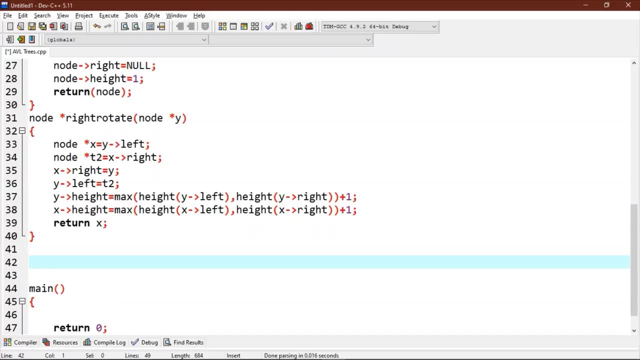 now return x. now return x. now return x. now let's write a utility function to left rotate subtree to left rotate subtree rooted with x. node bar left. rotate node bar left. rotate node star X. node star Y will be equals to XS right and node star t2 will be equals to XS. sorry, YS. 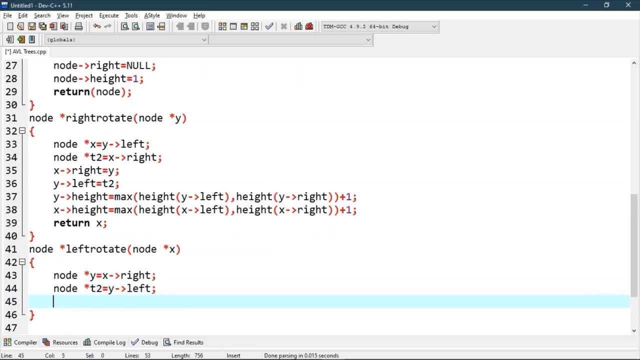 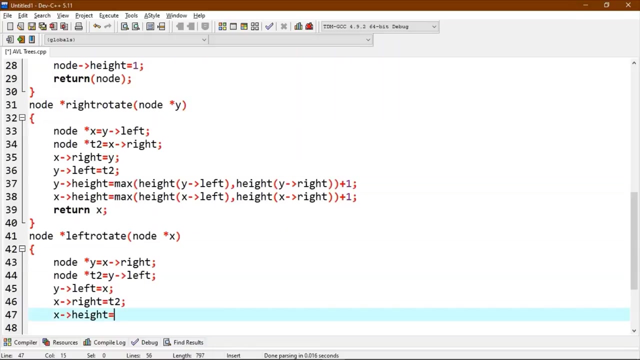 now we will perform rotation, so Y left will be equals to X and X right will be equals to t2. now let's update height. so X height is equals to maximum of height of XS left comma height of XS right and node star t2 will be equals to X and X right equals to maximum of height of YS left comma height of YS right. 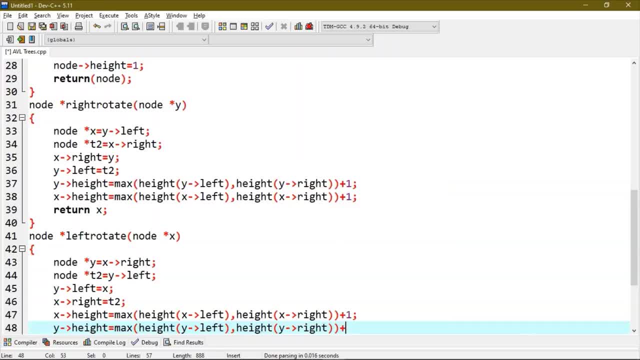 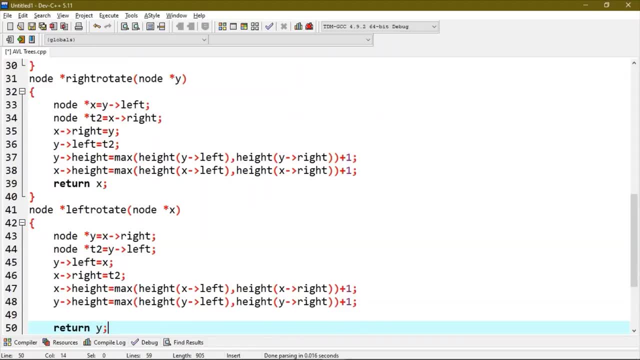 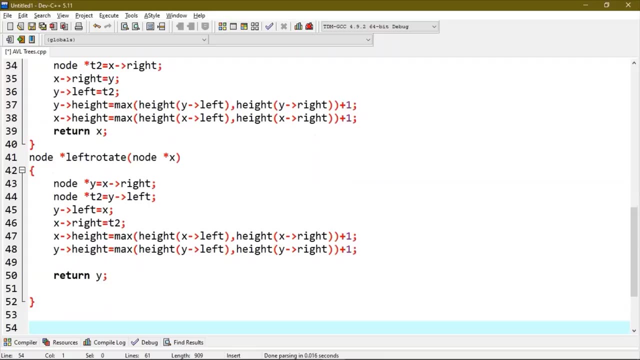 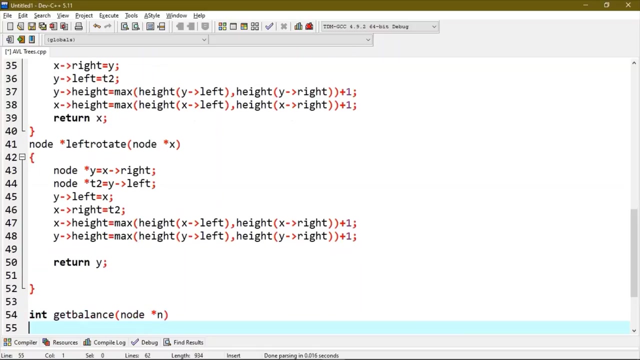 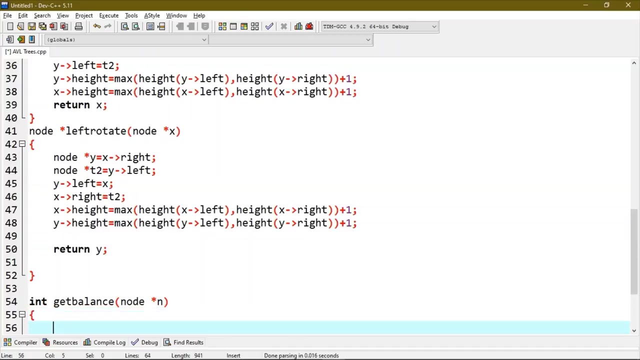 and node star t2 will be equals to X and X right comma height of YS, right comma height of YS right return Y. now let's write a function to get balance vector of node n, so int get balance argument as node pointer & if and is not n is equals to null, then we will. 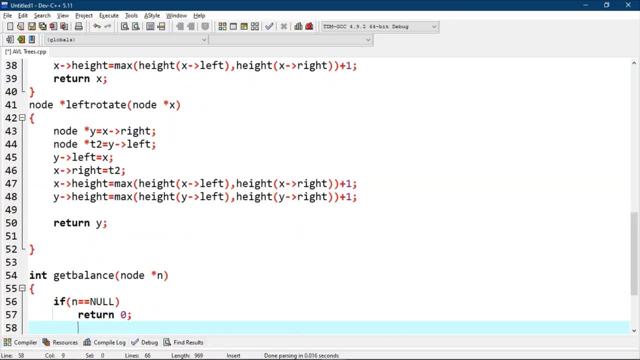 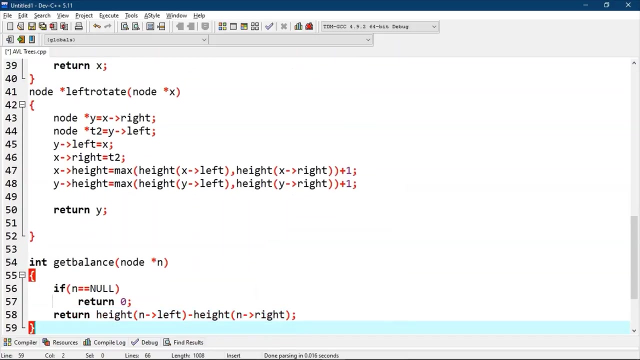 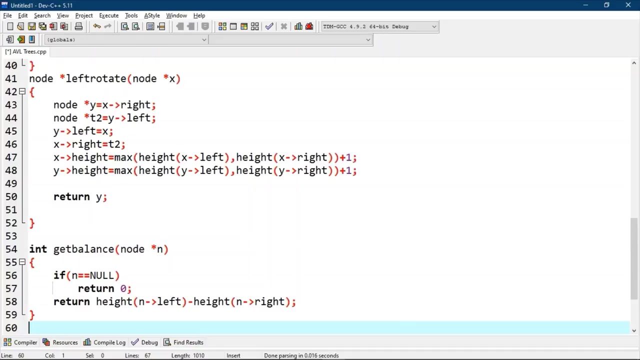 return. otherwise we will return height of n's left minus height of n's right. Now let's write a recursive function to insert a key in the subtree rooted with node and returns the new root of the subtree. So node star insert, node star, node comma int key. 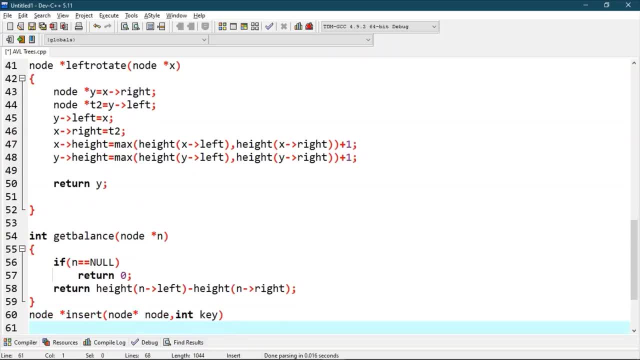 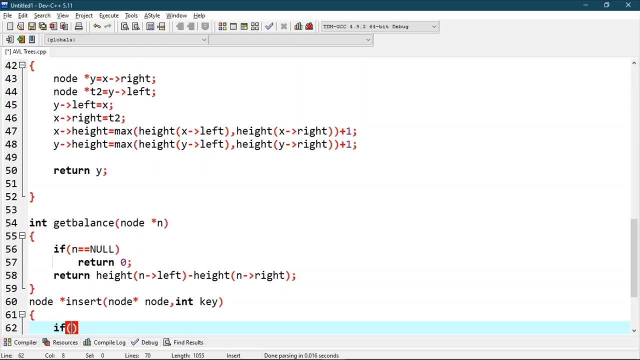 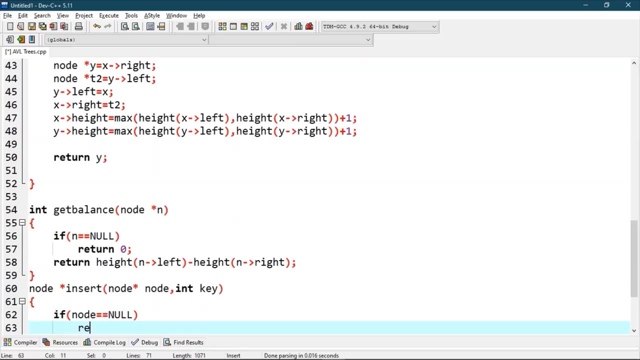 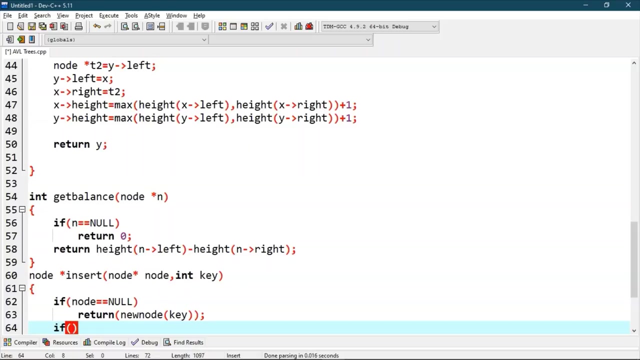 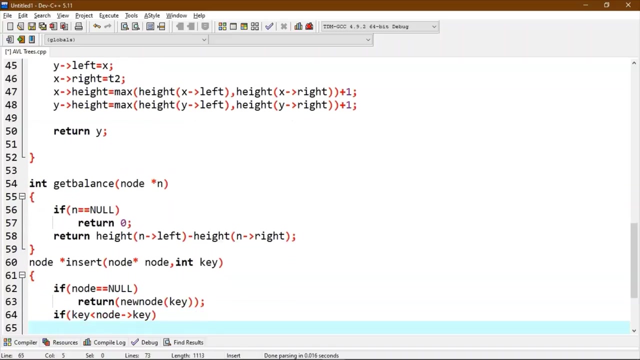 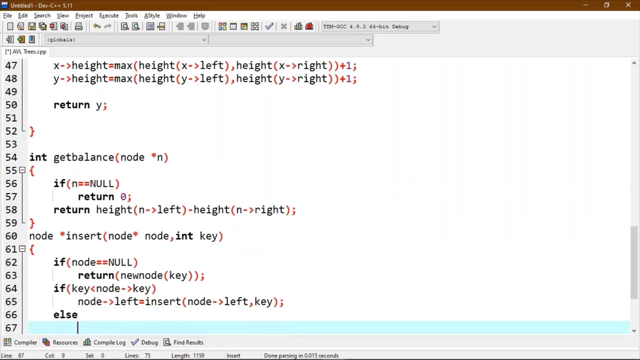 Now we will perform the normal BST insertion. So if node is equals to null, then we will return new node null int key. Now if this key is less than node's key, then node left will equals to int key. insert node left comma key. or else we will insert that in the right. 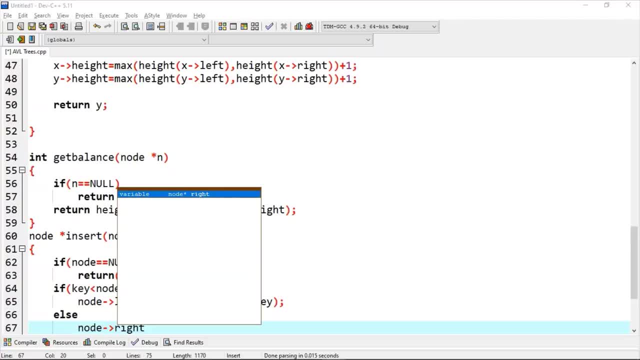 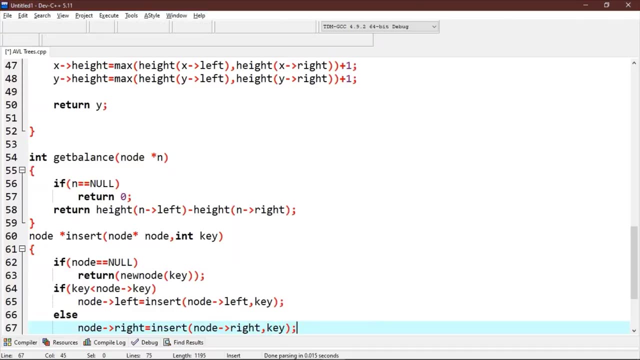 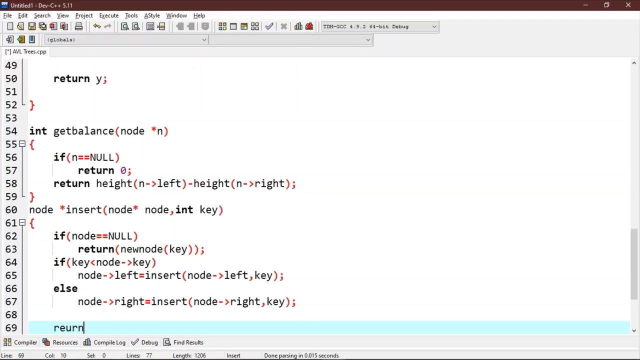 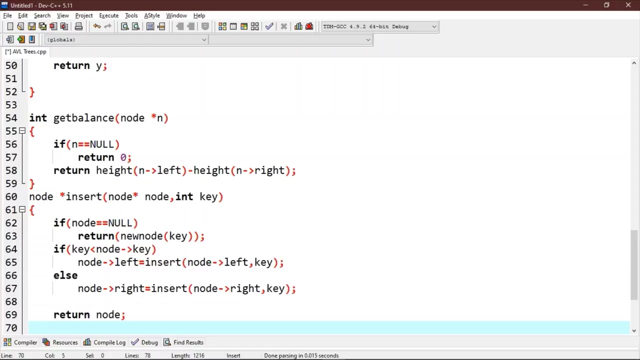 node right is equals to null. Now, if this key is less than node's key, Now we will return node. This, if else, will make sure that we will reach to the leaf node and then we will insert the key. Now we will update the height of this ancestor node. 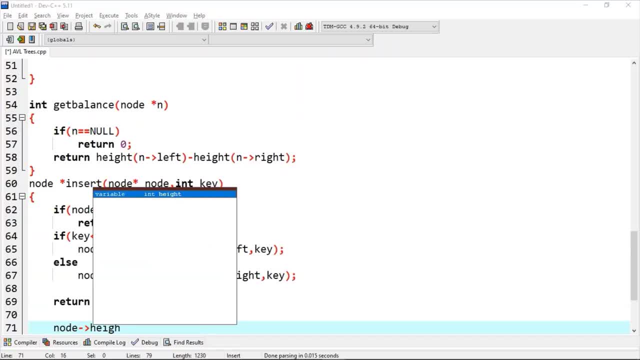 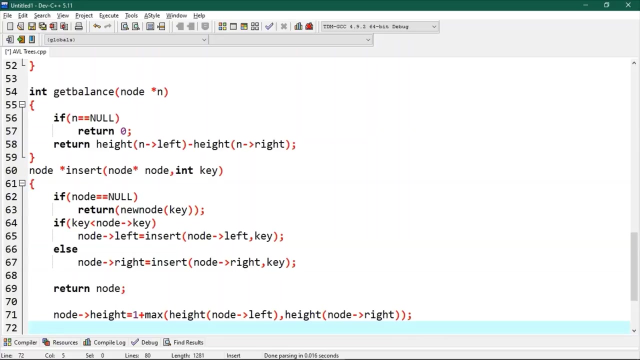 So node height is equals to 1 plus 2.. Max height of node: left comma height of node. right Now we will get the balance factor for this ancestor node to check whether this node became unbalanced. So int balance is equals to get balance. 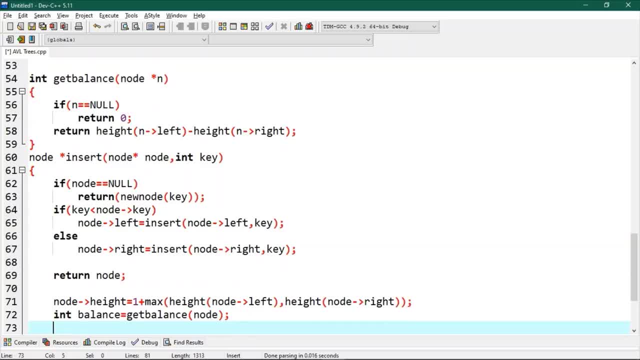 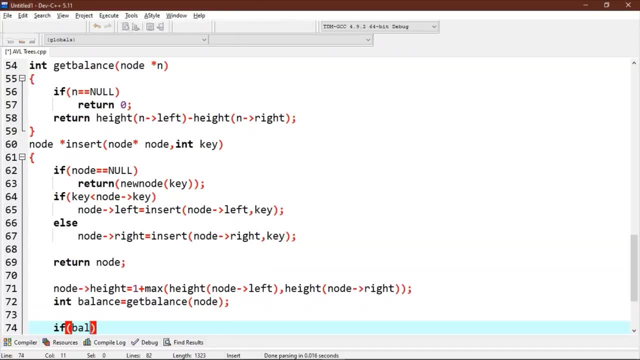 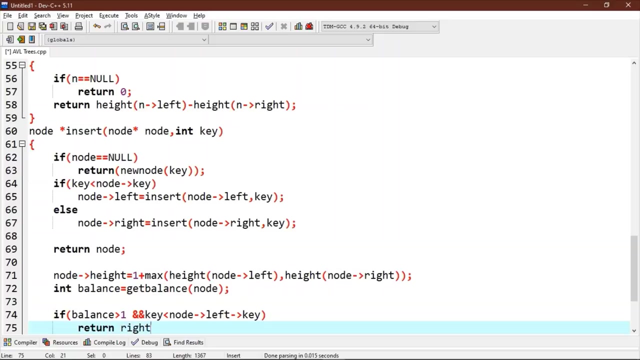 Now, if this node becomes unbalanced, then there are four cases. So if balance is greater than 1, and key is less than N. left key is higher than N, Then we will return. write rotate node. This is statement for the left left case or LL case. 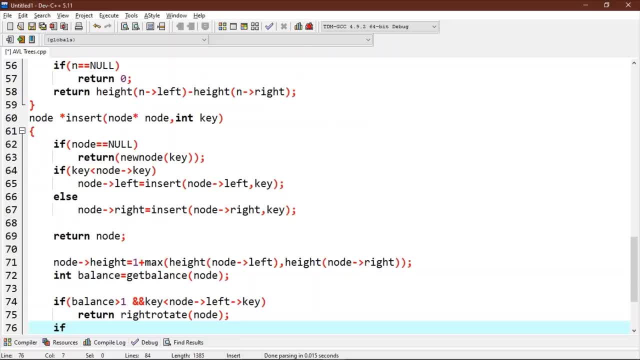 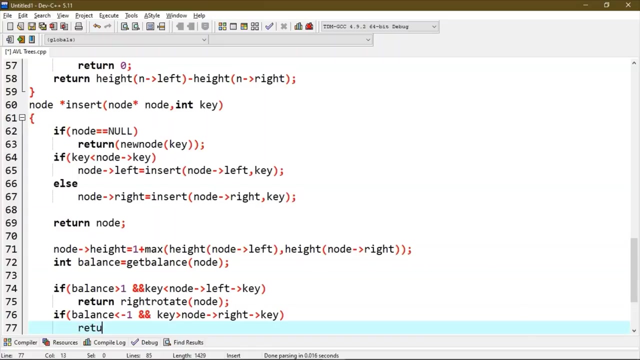 Now let's write it for the right right case or RR case. So if balance is less than minus 1.. And E is greater than node, Okay. So if balance is less than minus 1.. Then we will return left rotate node. 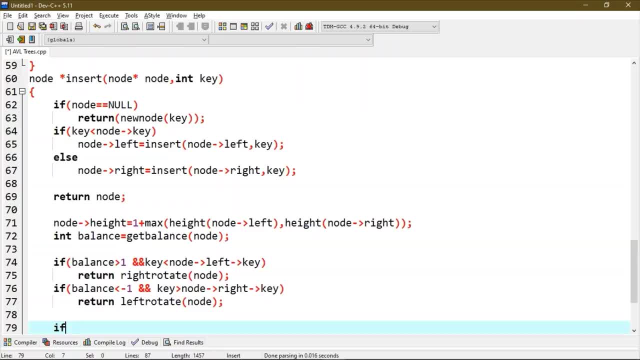 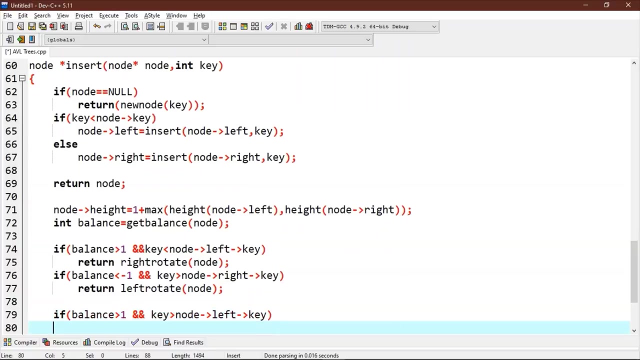 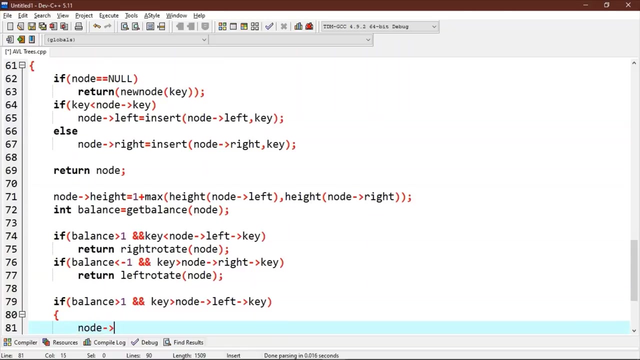 Now write for the left, right case or LR case. So if balance is greater than 1.. And key is greater than node Left key, Then node left is equals to left rotate node left. Now return right, left And E, So we will return left, left. 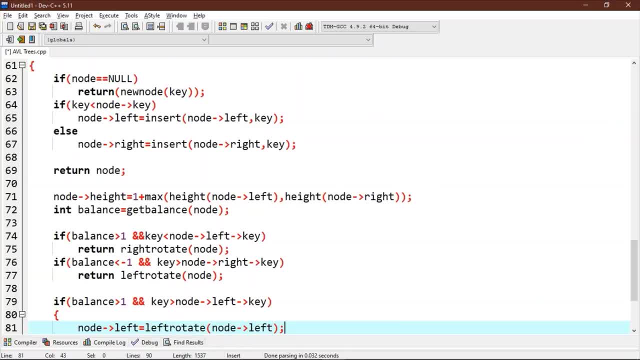 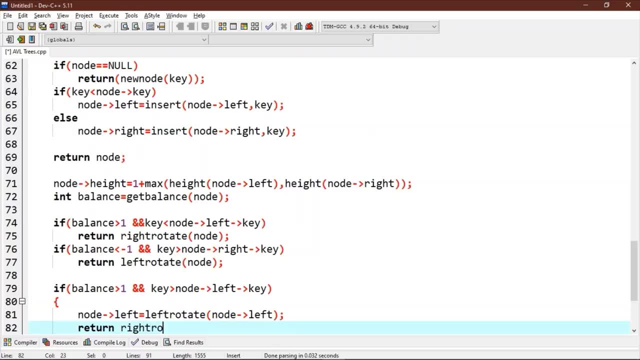 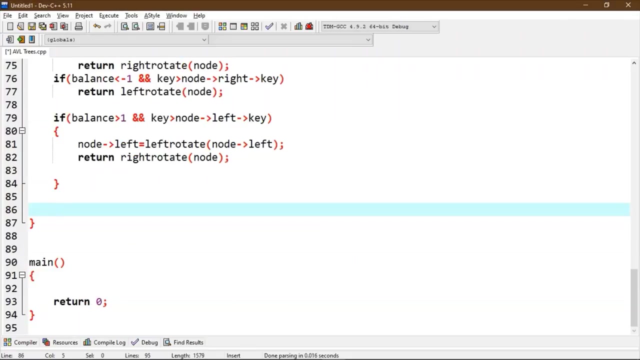 And E. So we will return left, left. Then we will return left, left And E. So we will return left, left And E. So we will return right right. Now let's write the right left case or RL case. So if 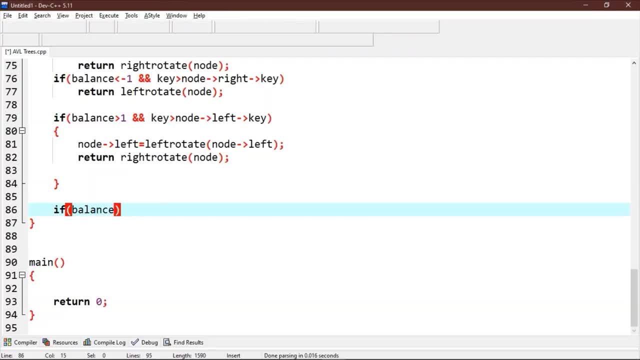 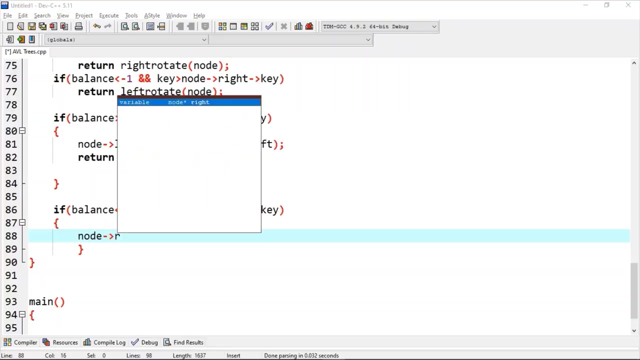 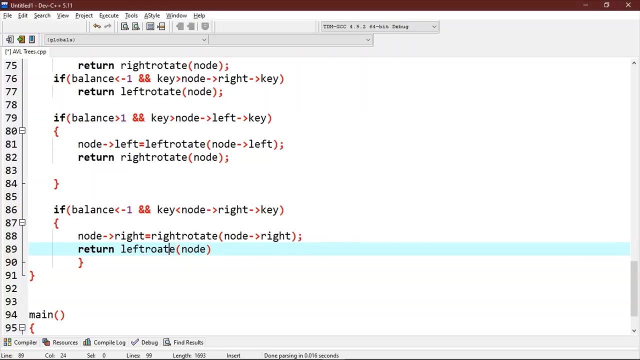 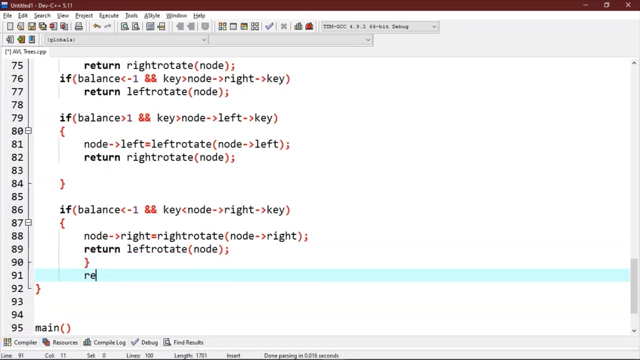 balance less than minus 1.. Yes, And key is less than node to the right. key and node right will be equals to right rotate node to the right and we will return left rotate now. we will return this node now. let's write a function to print pre-order traversal of this tree. 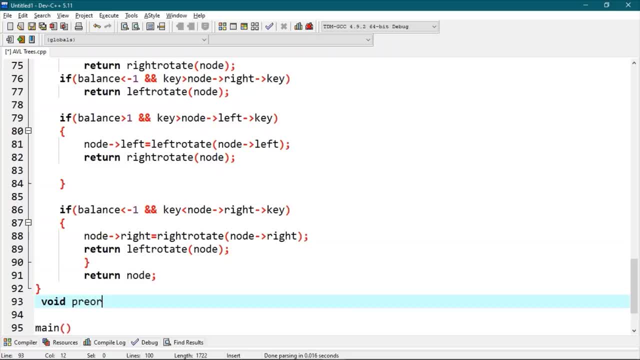 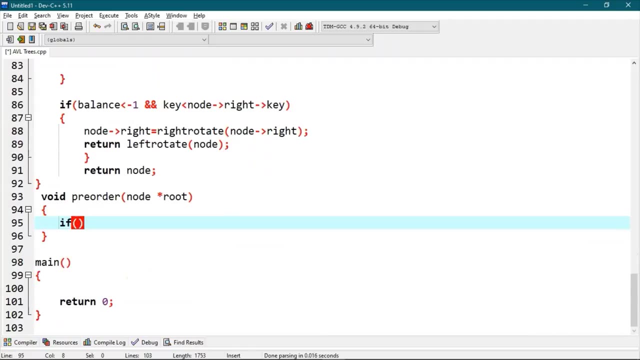 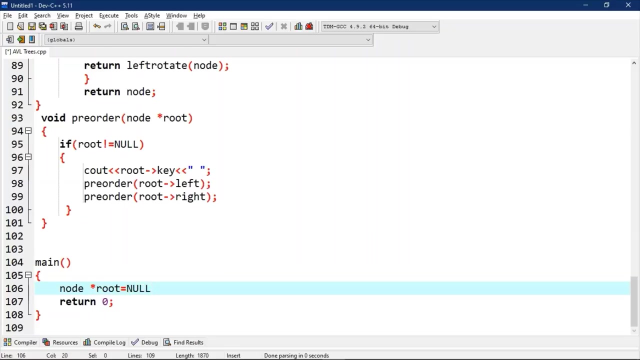 so void pre-order node star root. so now, if root is not null, then cout root key and now pre-order root and pre-order and pre-order node star root. now let's write the code for the main block. we will start with an empty tree. node star root is equals to null. 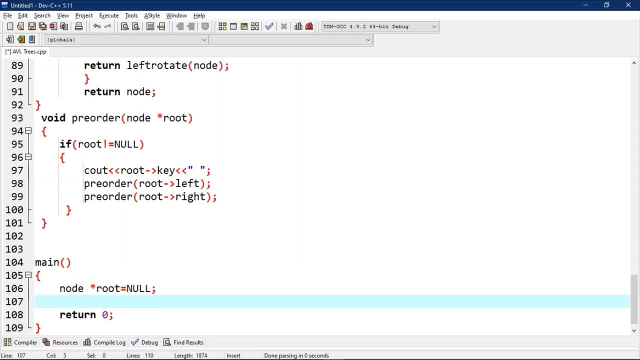 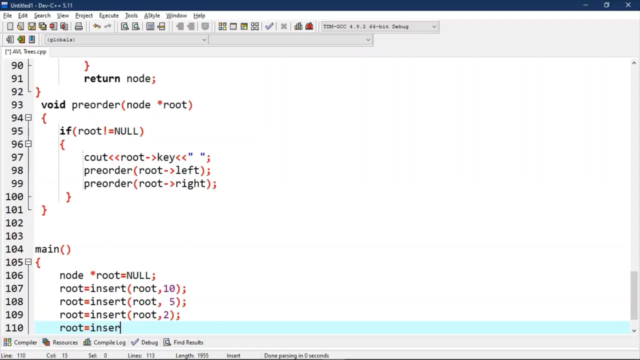 now we will try to construct tree. so root is equals to insert root. comma 10 now: root is equals to insert root. comma 5: root is equals to insert root. comma 2: root is equals to insert root. comma 3: root is equals to insert root. 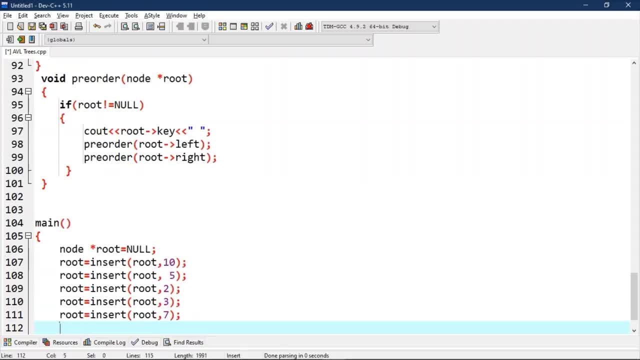 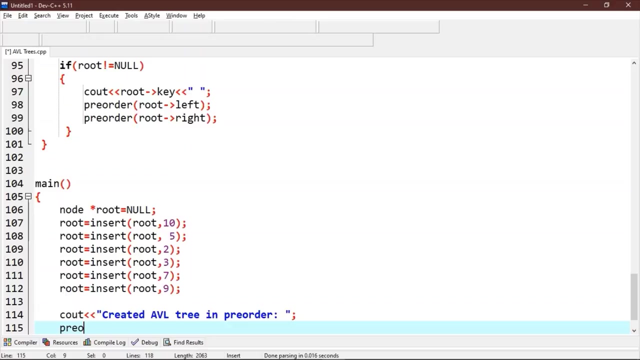 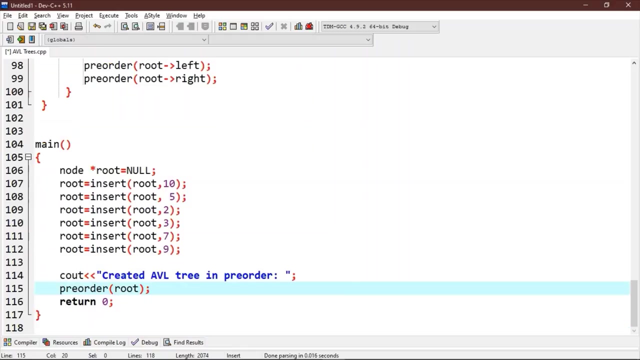 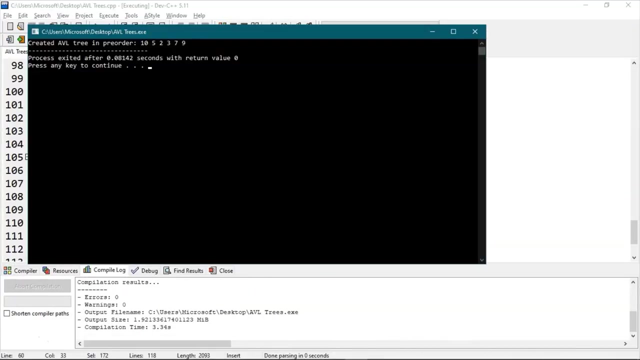 comma 7 and root is equals to insert comma 9. now let's try to print this tree. so cout 2 a. so how it works, is we exit? oh cab. so Let's execute this. As you can see, we have successfully created our first AVL tree. 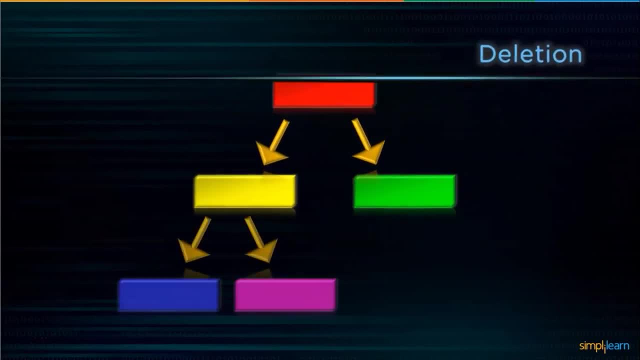 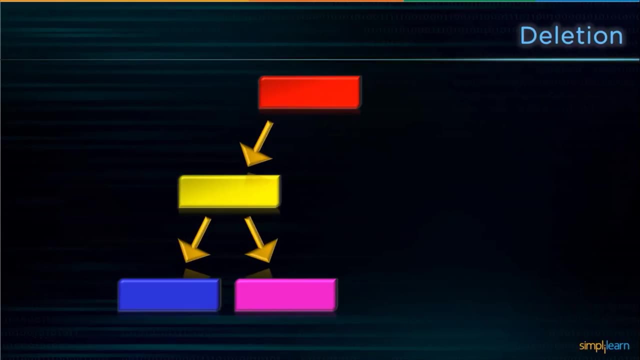 Let's get back to slides At last. deletion. We will delete a node following a binary search tree rules. Then we will check if all the nodes are balanced or not. If they are not, then we will balance it by using suitable rotations. 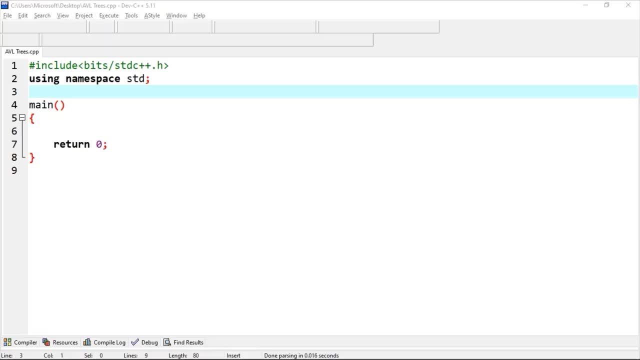 Now let's try these operations in a code editor. Let's start by creating a node. To create a node, we need a class node. We will define its members as public int key node star left node star right. int height. 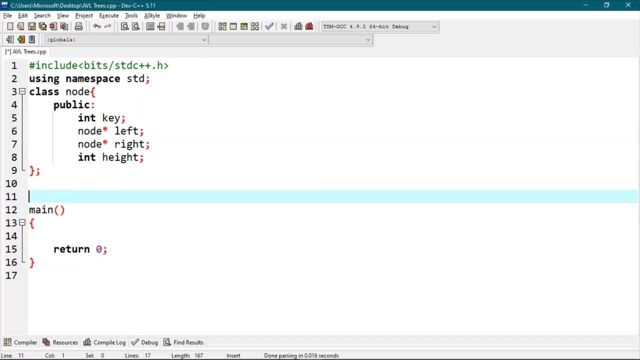 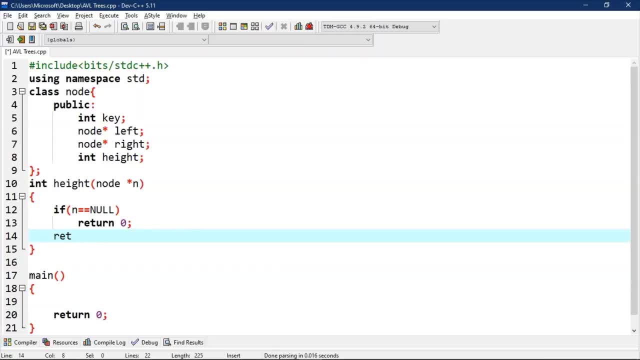 Otherwise we will return 0.. Now let's write a utility function to get maximum of two integer int max, int a, comma, int b. So we will return if a is greater than b, than a, else b. Now let's write a helper function that allocates a new node with a given key and null left and right pointers. 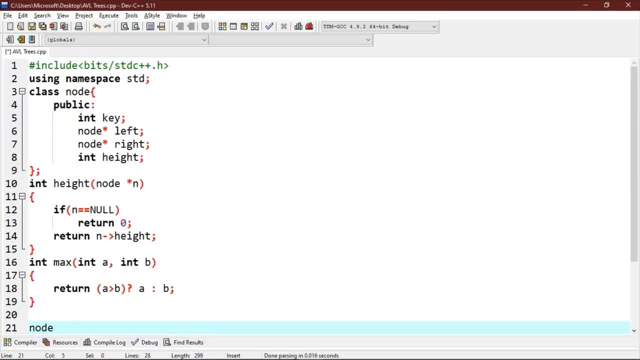 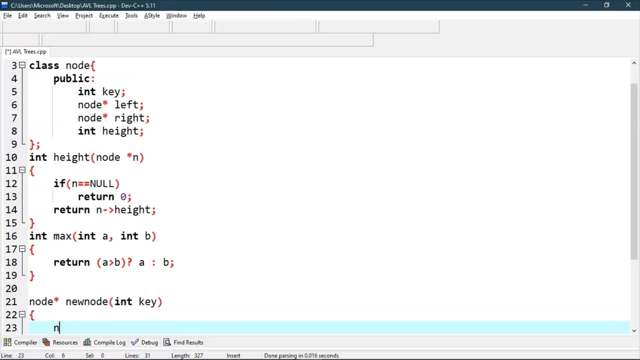 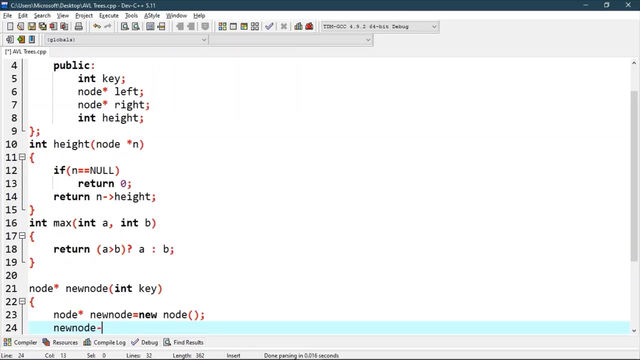 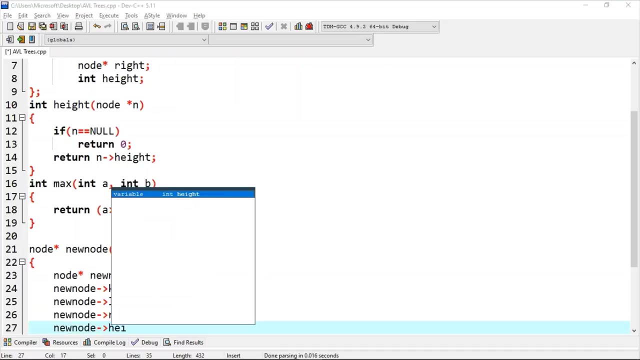 So node star, new node int key. So node star, new node is equals to new node. parenthesis on new node Videos. we'll get key as key. new node left is equals to null and new node right is equals to null. and new nodes height is equals to 1 because 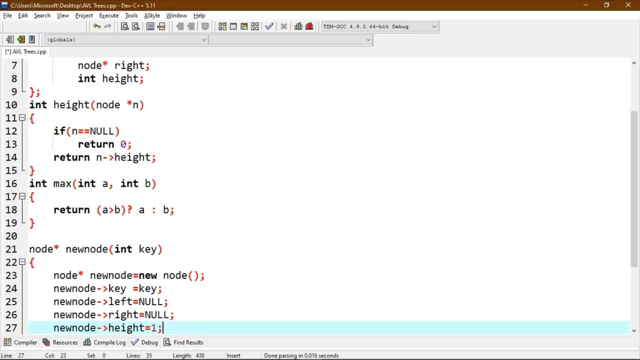 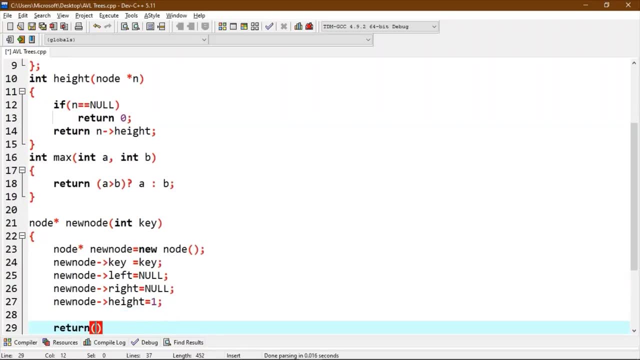 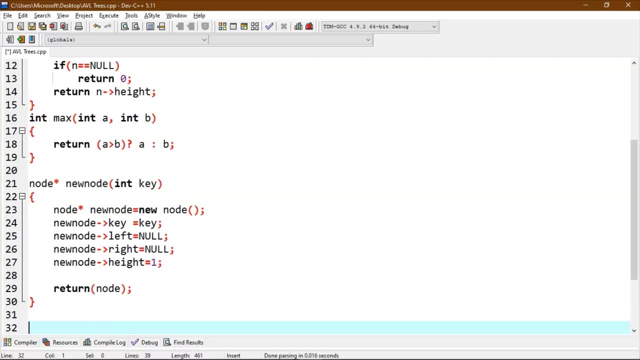 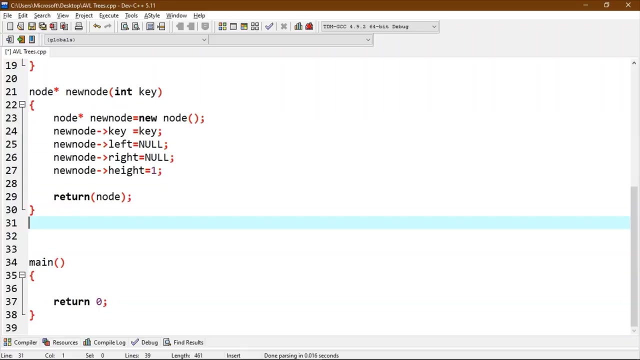 new node is initially added as leaf. that's why it is always be given as 1. now we will return this node. return node. now let's write a utility function to right rotate a sub-tree rooted with y. so node are: right rotate node. right rotate node. 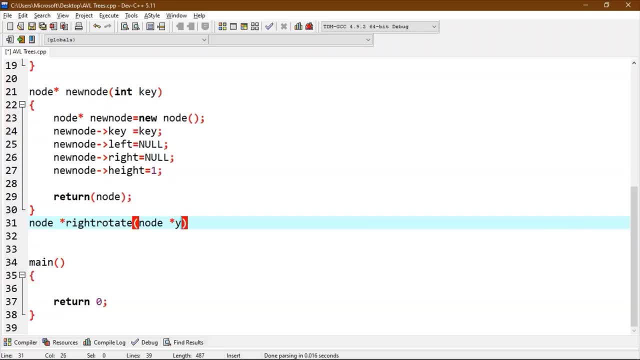 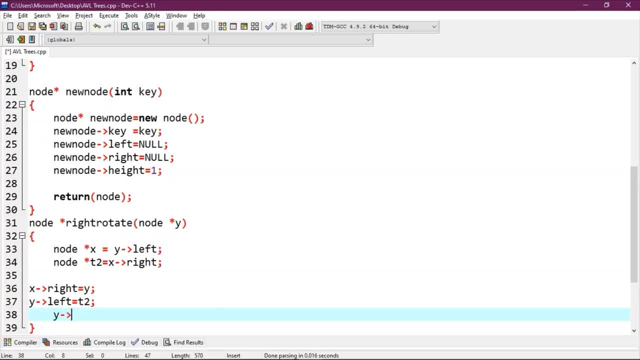 Now we will update heights, so y height is equals to maximum of height of y left comma. height of y right plus 1 comma. height of y right plus 1 and x height is equals to maximum of height of x's left comma, x's right plus 1. 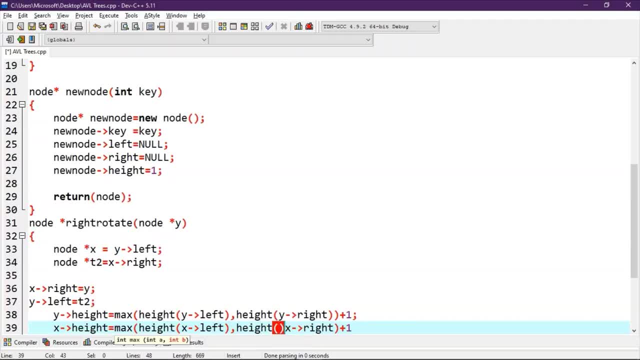 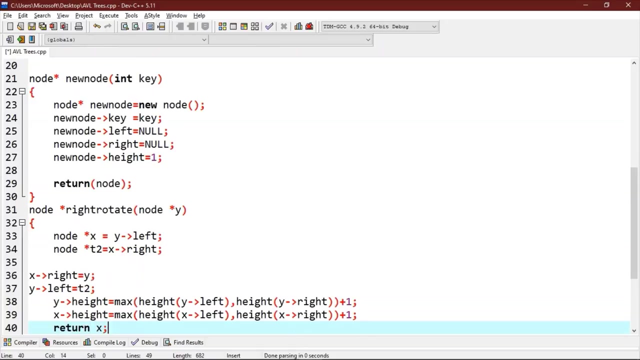 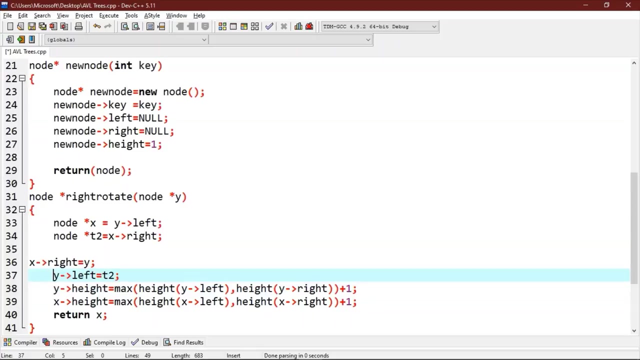 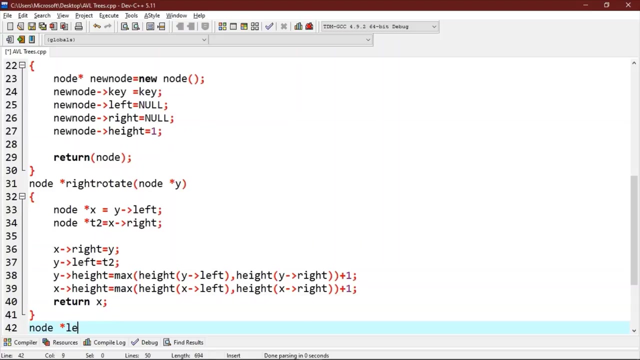 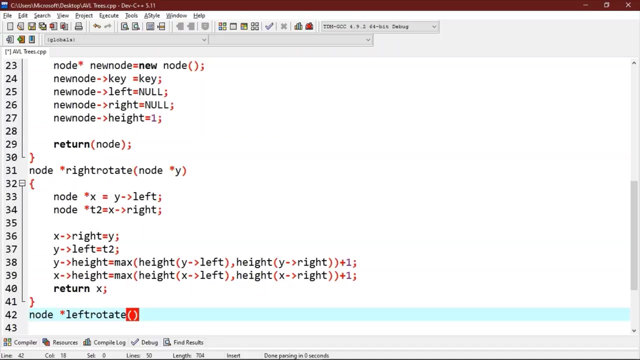 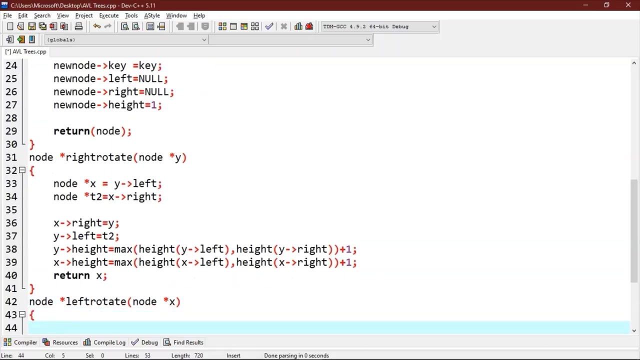 comma height of y right plus 1 comma height of y right plus 1 comma height of y right plus 1. Now we will return this new root. so return x. Now we will return this new root, so return x. Now we will write: node star left: rotate node star x. node star y will be equals to: 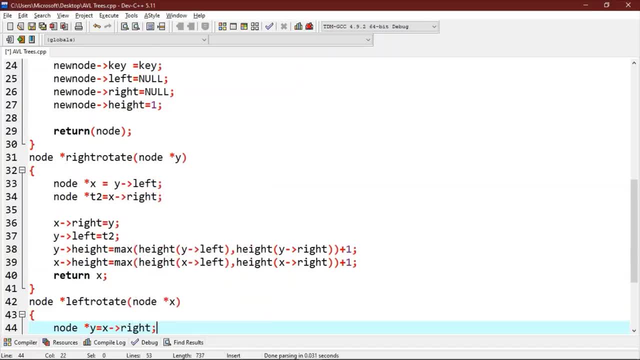 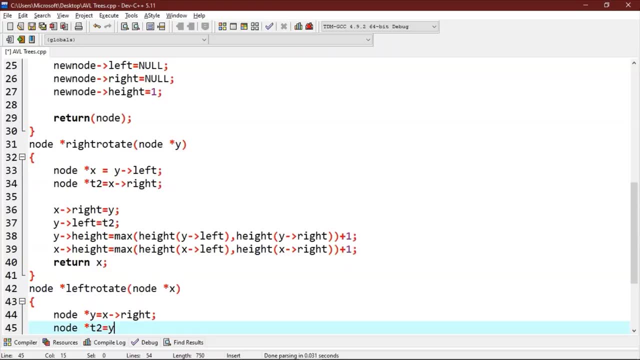 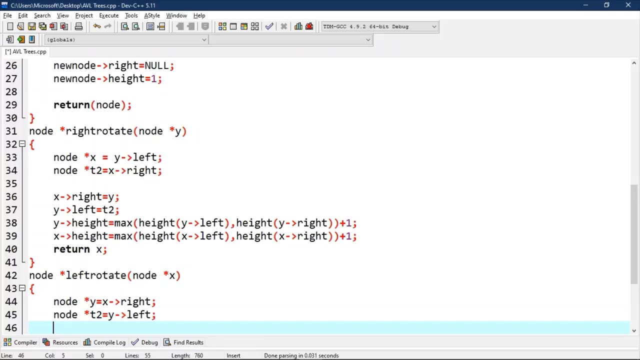 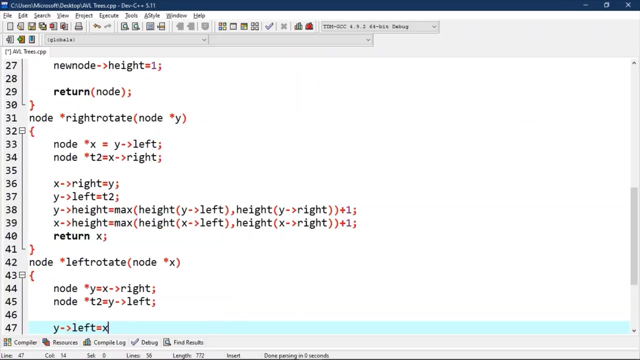 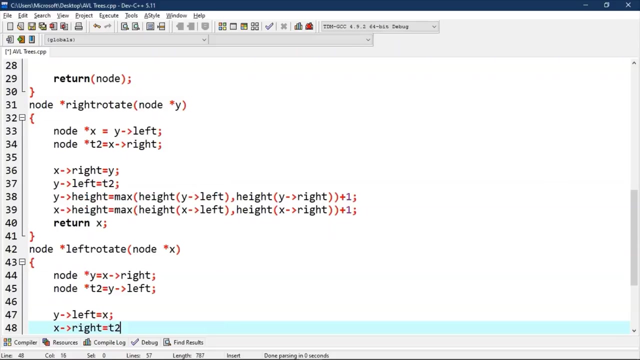 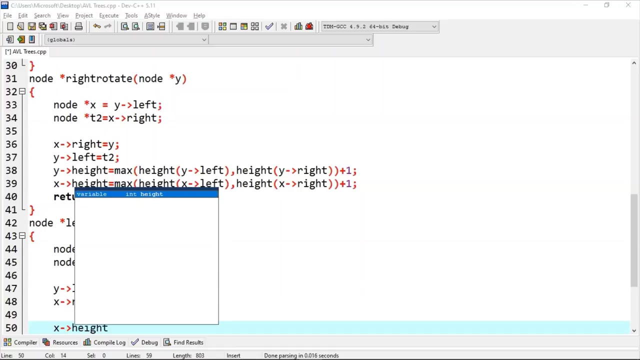 x is right and node star t2 will be equals to y is left. Now we will perform rotation, so y left equals to x and x right is equals to t2.. Now we will update these heights, so x height is equals to maximum of height of x left. 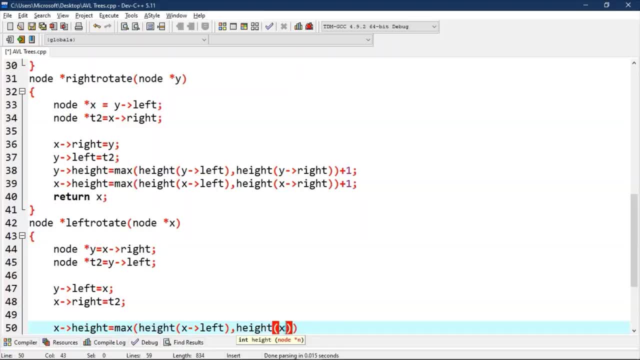 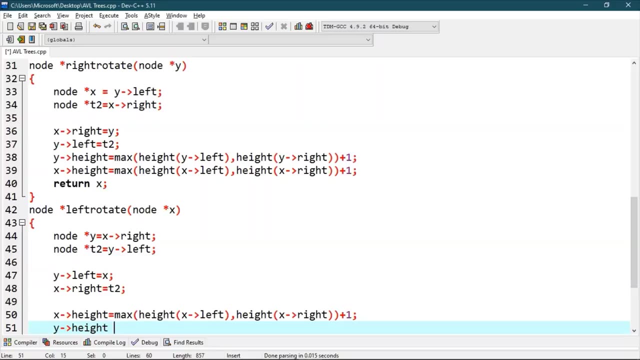 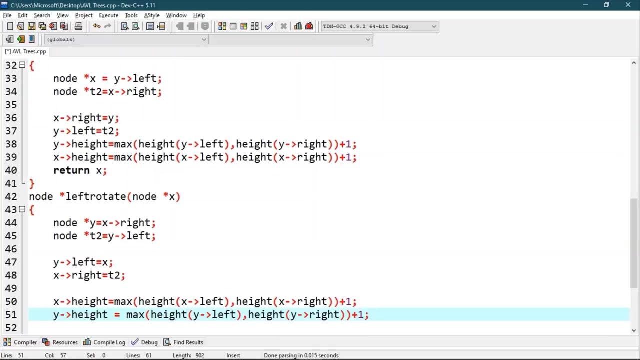 comma. height of x right plus 1 and y's height is equals to max of height of y's left comma. height of x right comma. height of y's left comma. height of y's right plus 1.. Now we will return this y. 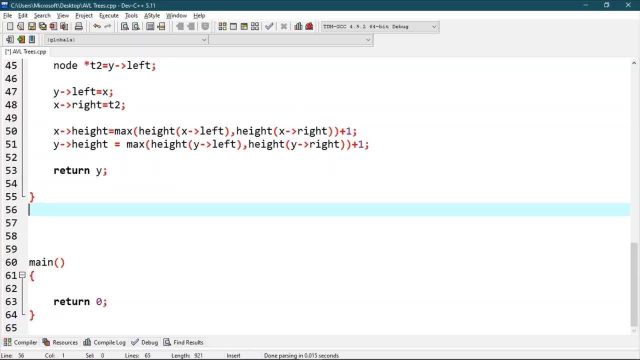 Now we will write a function to get balance factor of node n. Now we will write a function to get balance factor of node n. So int int get balance node star n. int get balance node star n. So int get balance node star n. 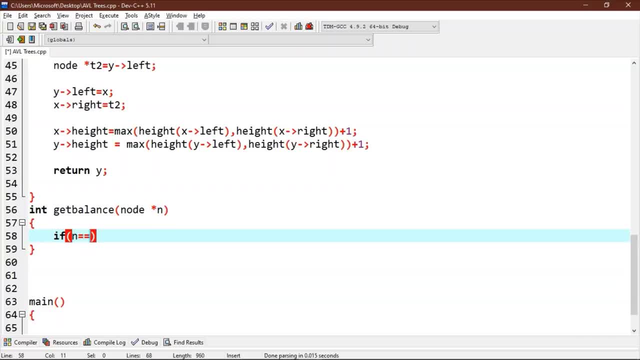 If is equals to null, we will lost. If is equals to null, we will lost. then we will return 0.. If is equals to null, we will also need to return zero. Otherwise, if x is 0, we can change to minus 1. 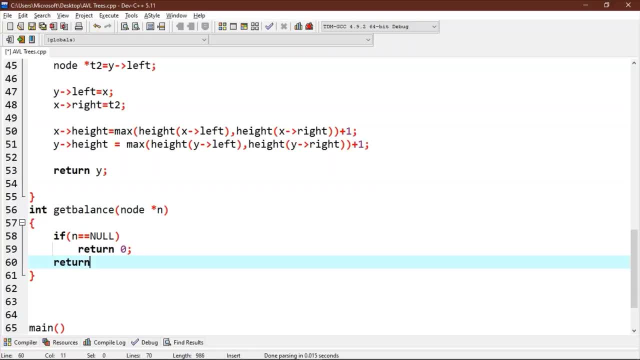 Otherwise we will return height of n's left minus height of n's right. Now let's write a function to insert a node, So node star. insert So node star, node comma int key. Now we will perform normal BST rotation. So if node is equals to null, then we will return new node key. 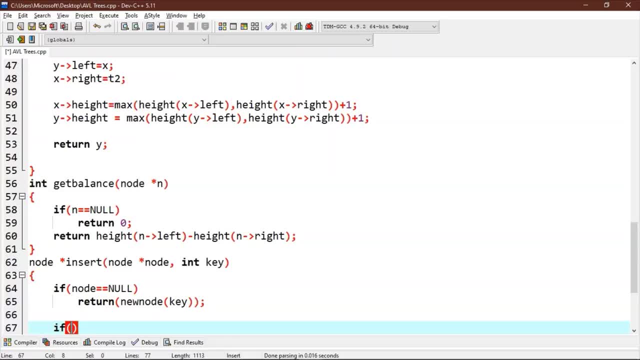 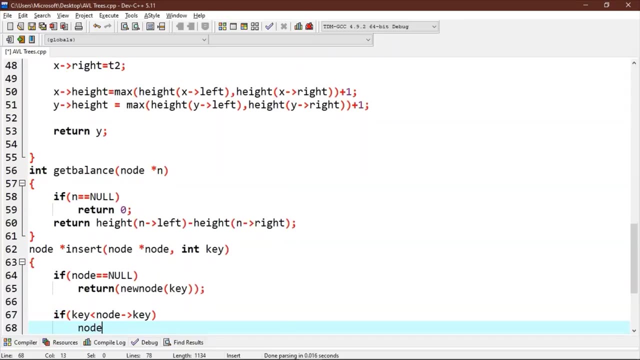 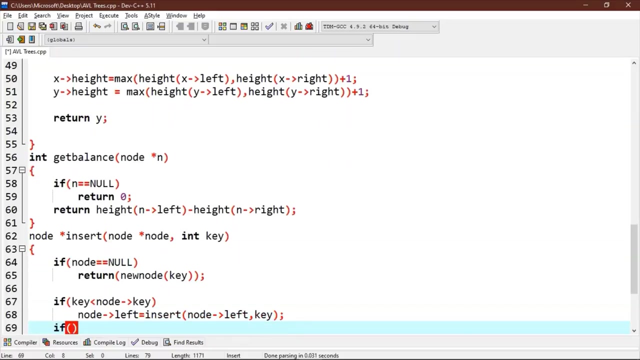 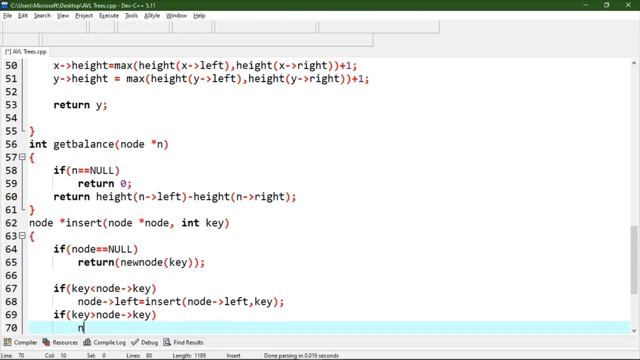 So now, if key is less than node key, Okay, Then node left will be equals to insert node left comma key. Okay. If node key is greater than node key, then node right is equals to insert node left comma key. Write comma key. 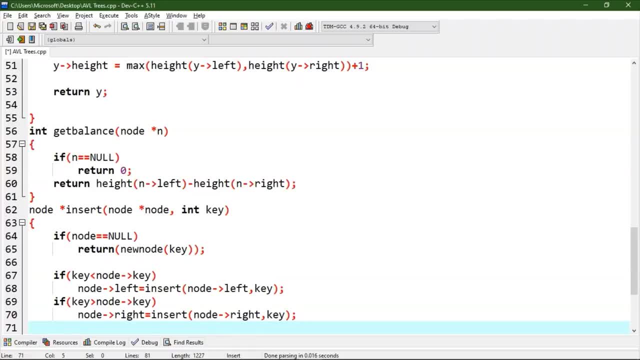 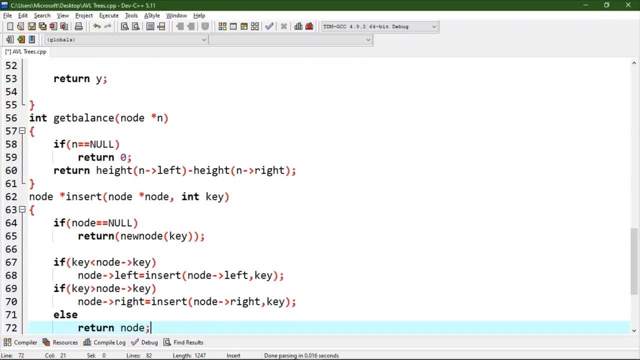 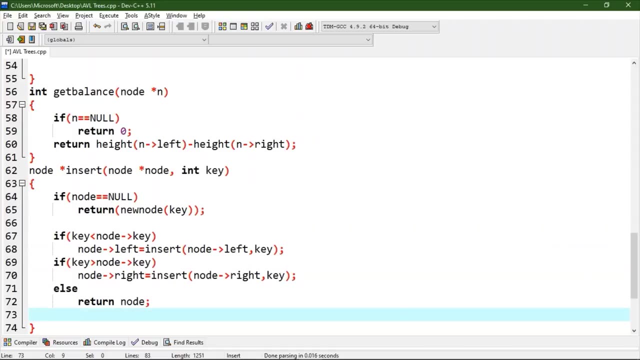 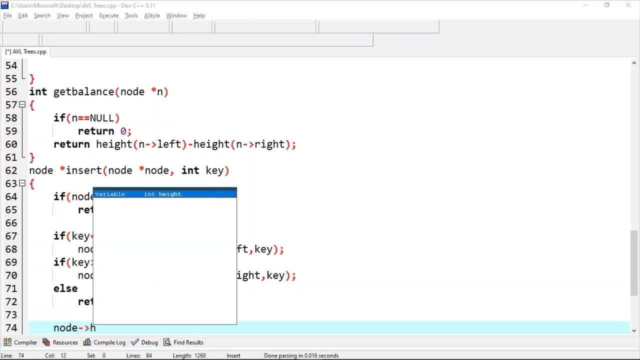 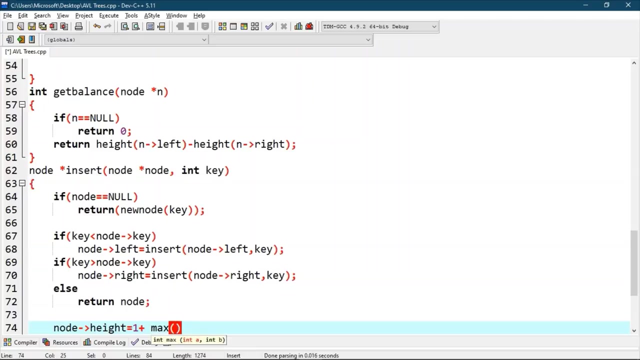 Else we will return node because equal keys are not allowed now. we will update the height of the ancestor node, so node height goes to 1 plus max height of node. left comma height of node. right now we will get the balance vector of this ancestor node. 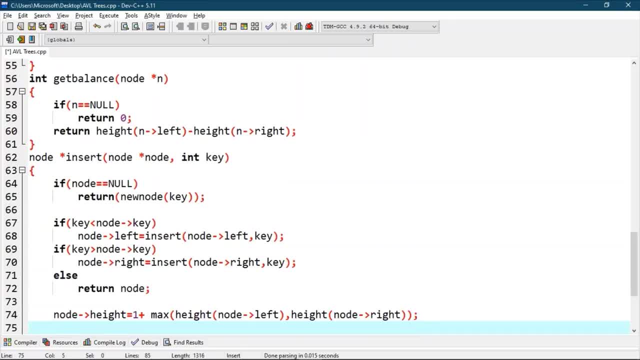 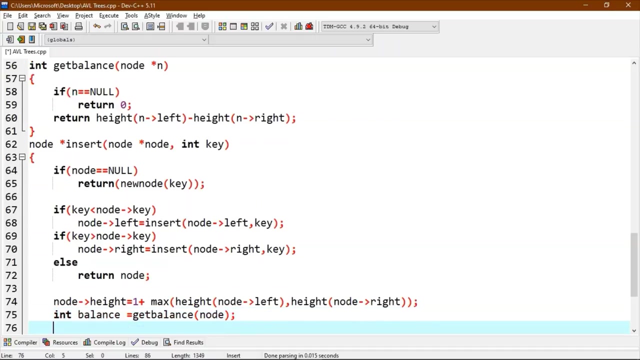 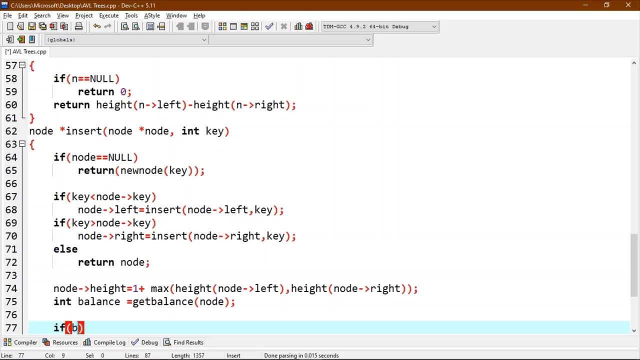 to check whether this node becomes unbalanced. so if so, int balance equals to that balance of this node. now, if this node becomes unbalanced, then there are four cases that could be possible. first up ll case. so if balance is greater than 1 and key is less than node left, 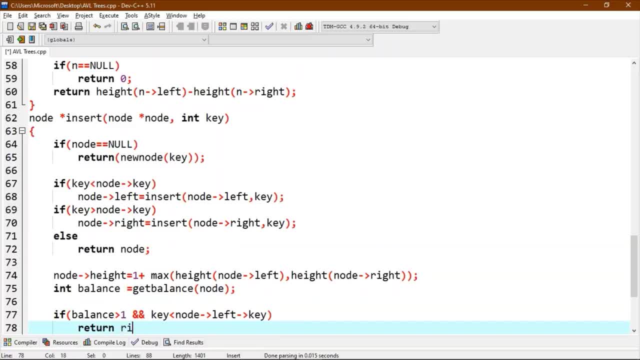 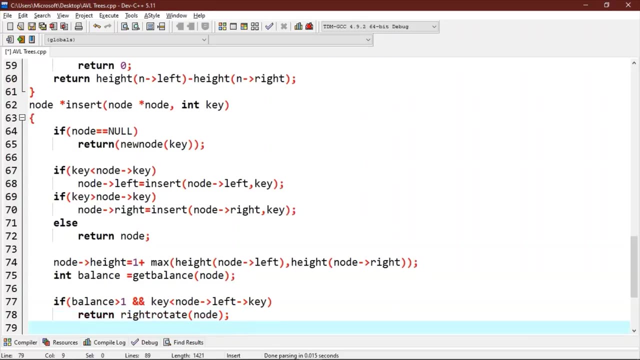 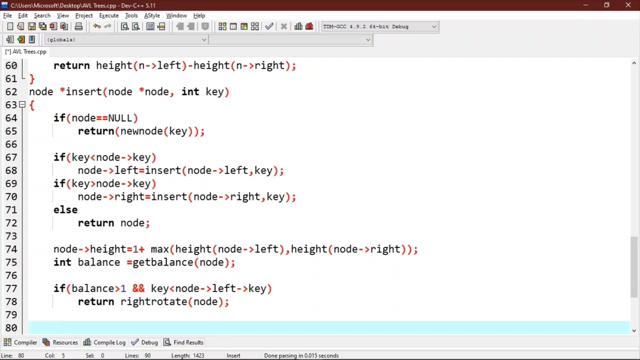 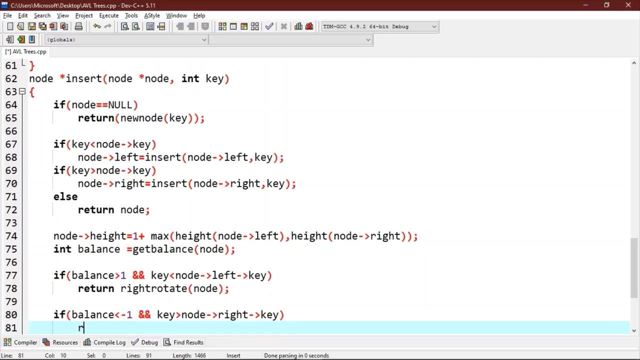 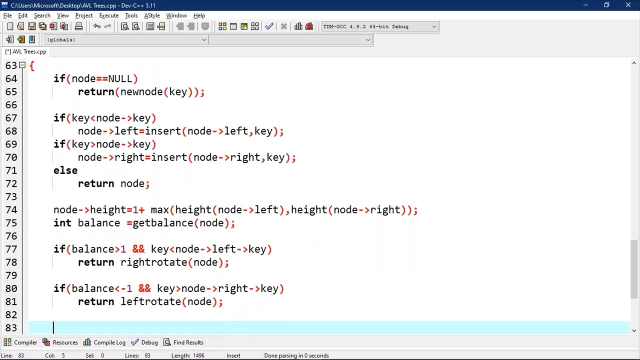 return right rotate and now brown case. now let's write right right case. so if balance is less than minus 1 and key is, then we will return leftRotateNode. now let's write leftRight case. so if balance is greater than 1 and key is greater than 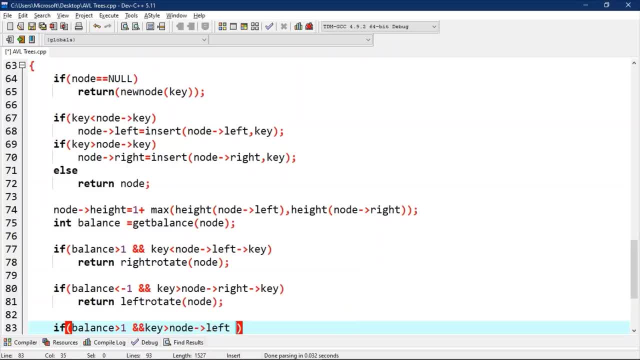 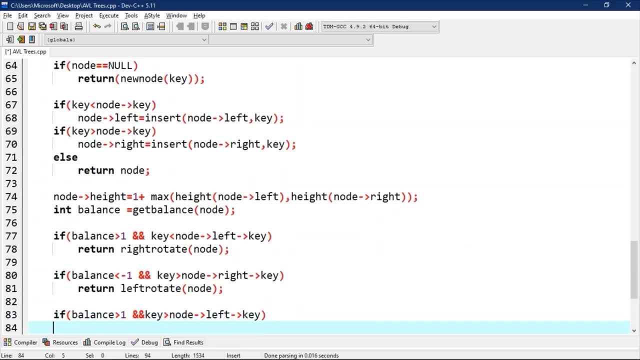 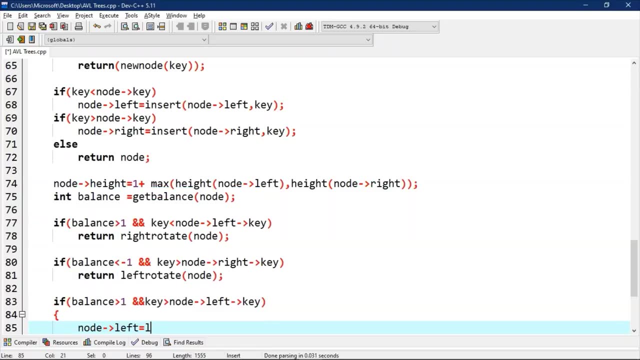 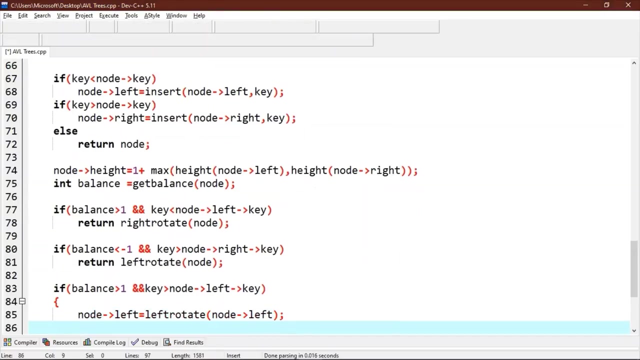 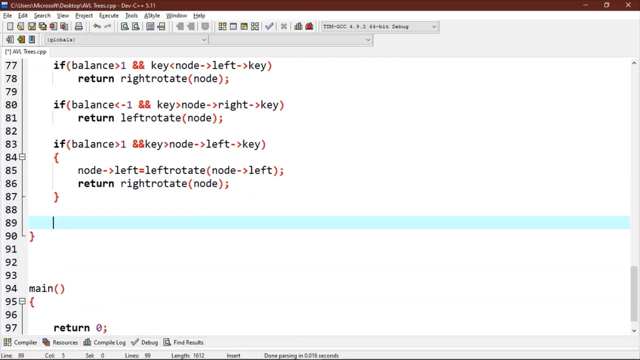 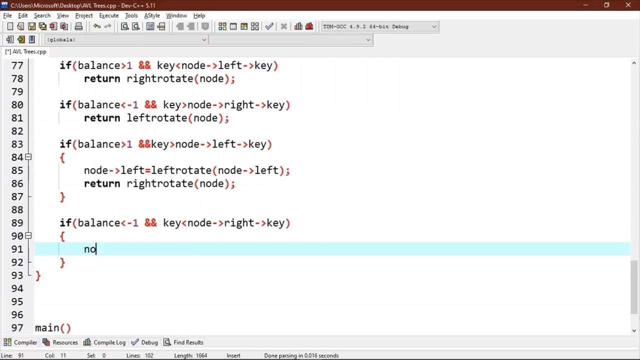 nodeLeftKey, then node left will be equals to left rotate node and we will return right rotate node. now let's write the case for right left case: if balance is less than minus one and e is less than node right, so node right is equals to right rotate. 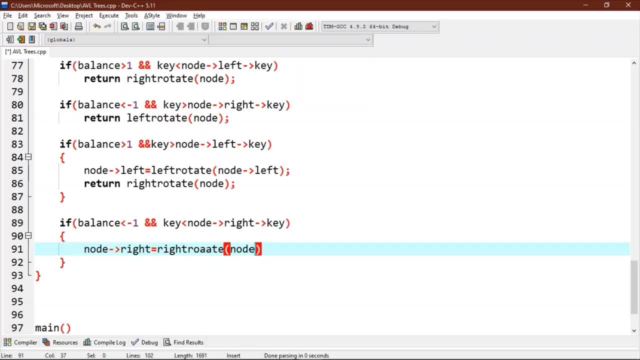 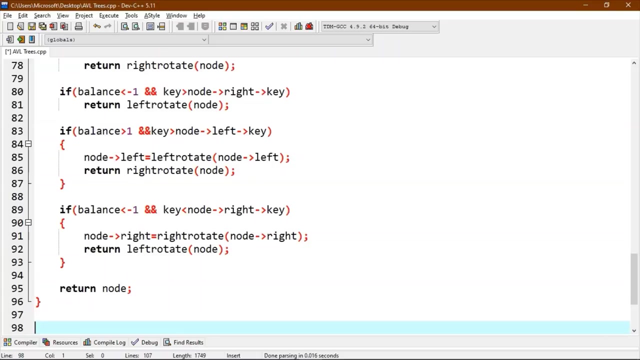 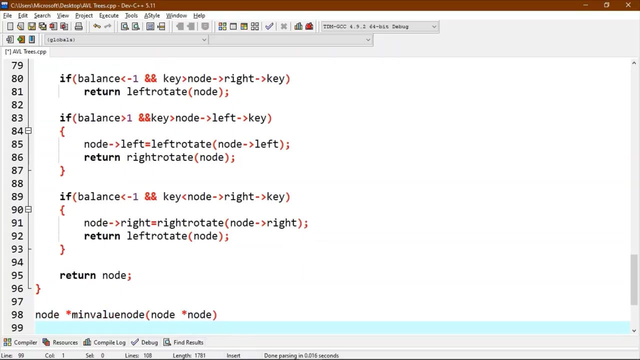 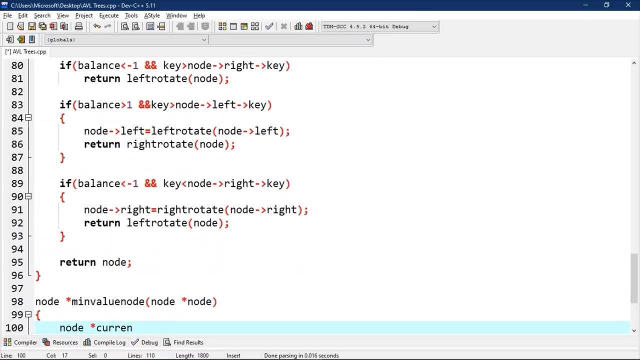 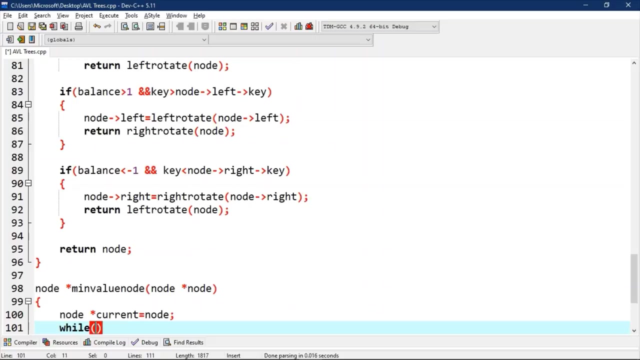 node. right now we will return left rotate node. now let's return the unchanged node pointer, so return node now. let's write a function to find when: minimum value node, so node star. min value node- node- star node, so node star. current equals to node. so while we return current, left is not equals to. 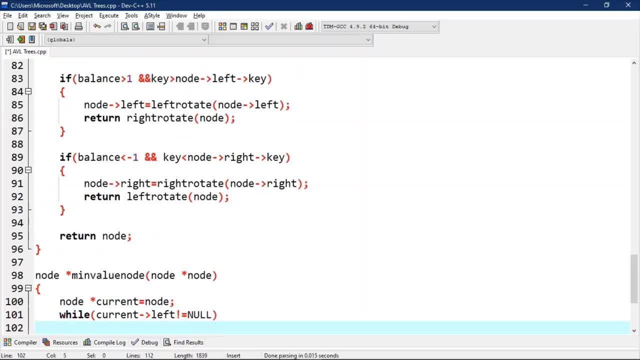 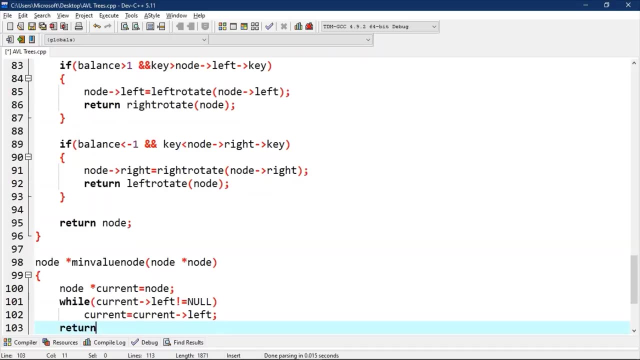 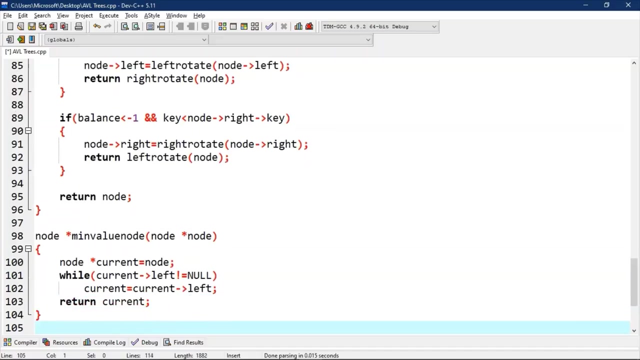 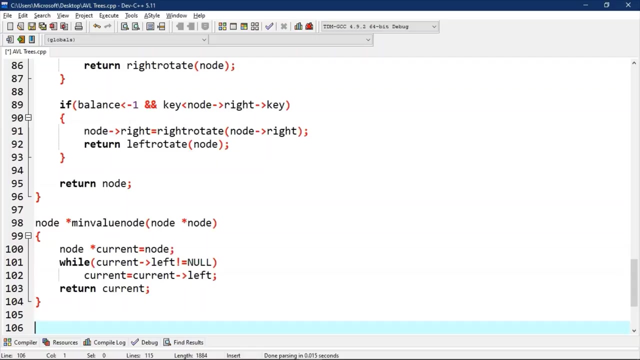 null. current is equals to current at left. now we will return current. left is not equals to null. now we will write a recursive function to delete a node with the given key from subtray with the given root. so node star: delete node. its arguments are node pointer root. 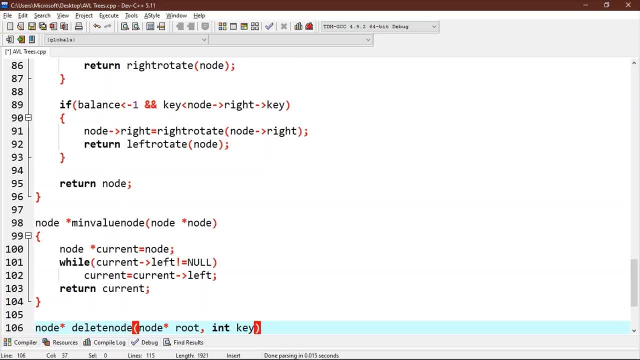 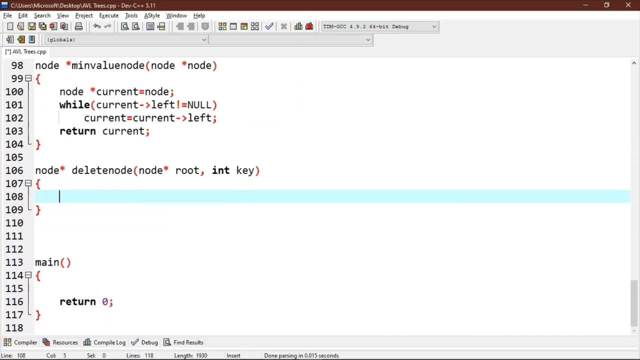 comma int key. for starters we will perform standard bst delete. so if root is equals to null, then we will return root. root is equals to null, then we will return root. root is equals to null, then we will return root our tree. so characters under the axis boundary. 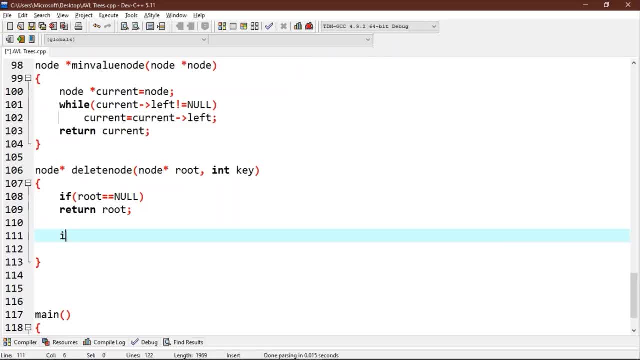 means we will return root. if the key is smaller than the root key, then it lies in the left subtree. so if e is less than root e, then you will surely get the root value. okay, so if you have a segment known as rootMotor, then we will write the rootMotor to the root window. 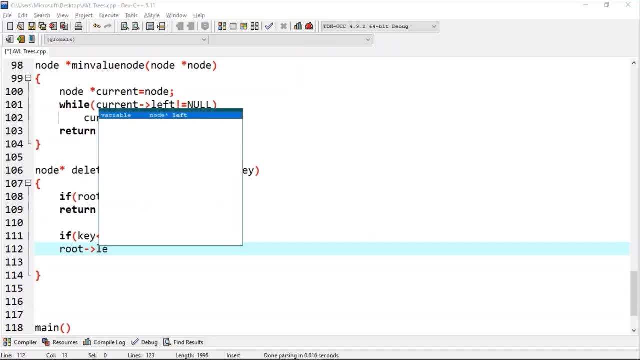 Then root left will be equals to delete node root to the left comma key. Now if key to be deleted is greater than the root key, then it lies in the right subtree. So else, if key is greater than root key, then 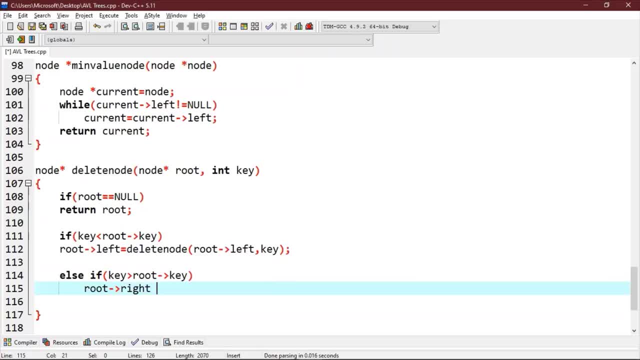 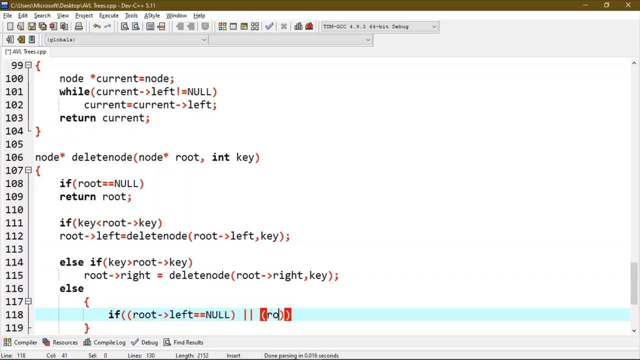 root right equals to delete node root right comma key. Now, if the key is same as the root key, then this is the node to be deleted. So else, if root left equals to L R, for déjà vu, use the semicolon 没有. 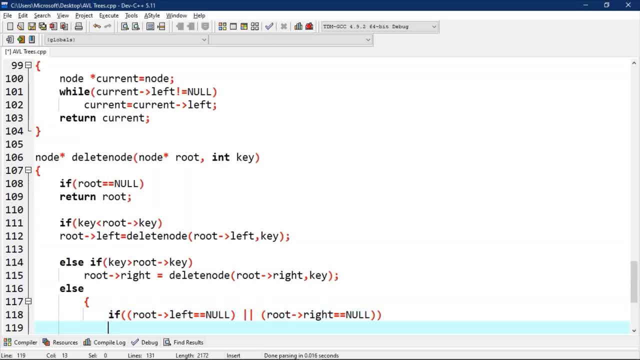 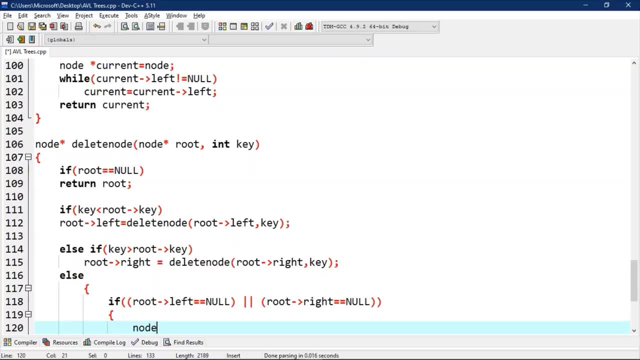 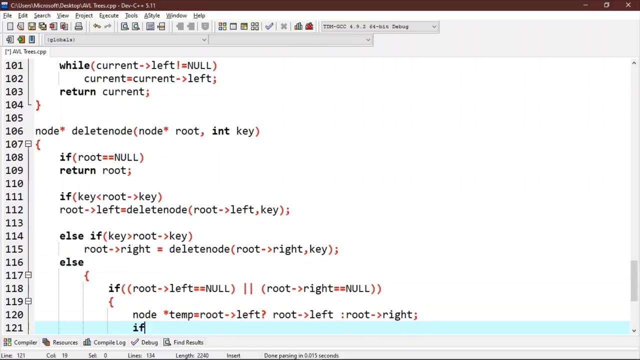 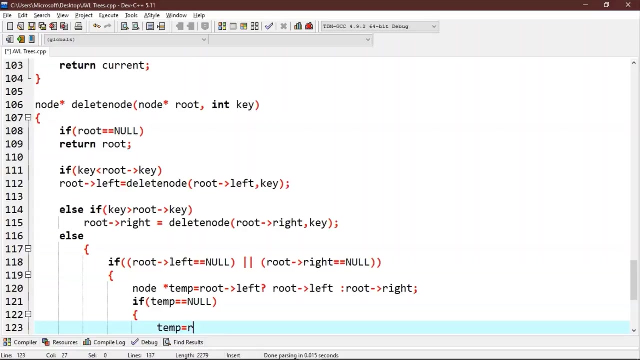 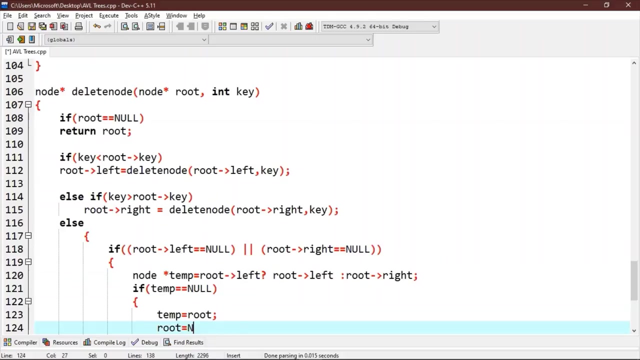 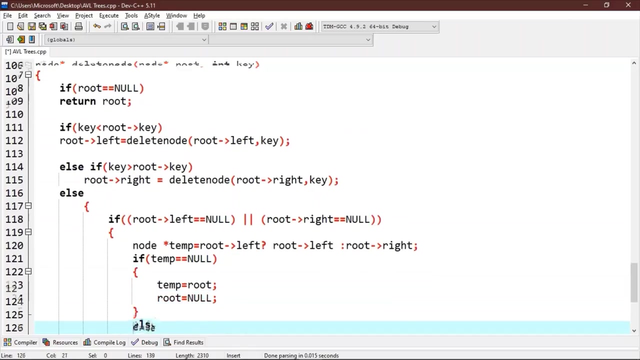 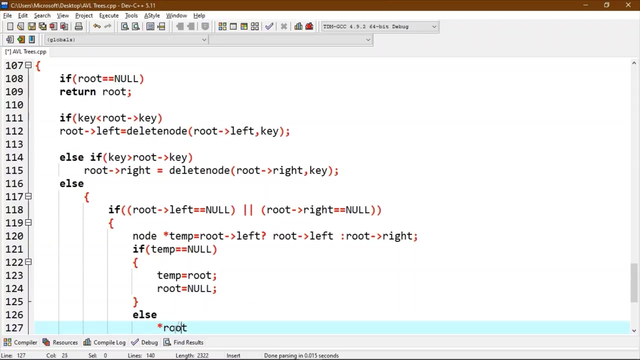 but the, but the but must to have readily to keep save. save for ok and a. do security vi to root. left now f temp is equals to root, then temp will be equals to root and root will equals to null. else root will be equals to star. 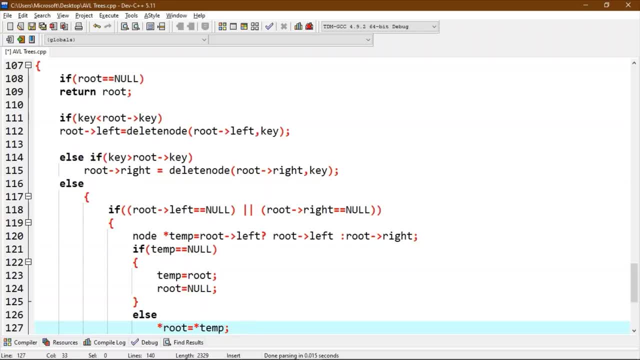 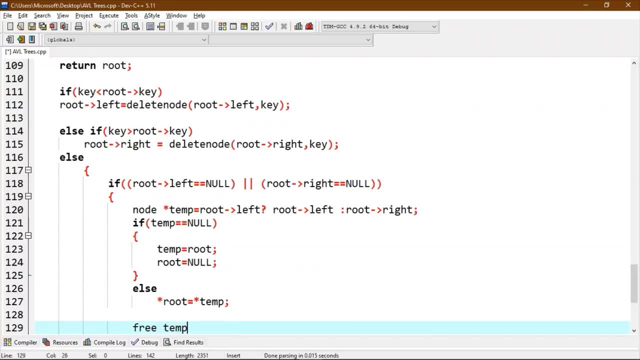 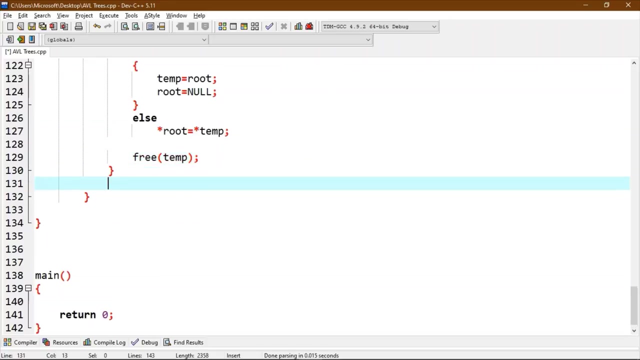 temp and free temp. let's, let's, let's, let's, let's simpler, let's, let's, let's lower this. ok, so input new node: start temp is equals to min value node root. right now we will copy the inorder successor with interpretations in order successor here: 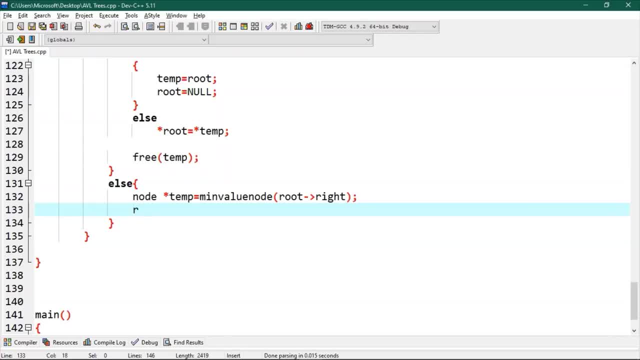 let's inorder successors data to this node. so root E is equals to temp key now we will delete this inorder successor. so root write is equals to delete node root comma temp key now. if root is equals to null, then we will return root. now we will update the height of the current node. 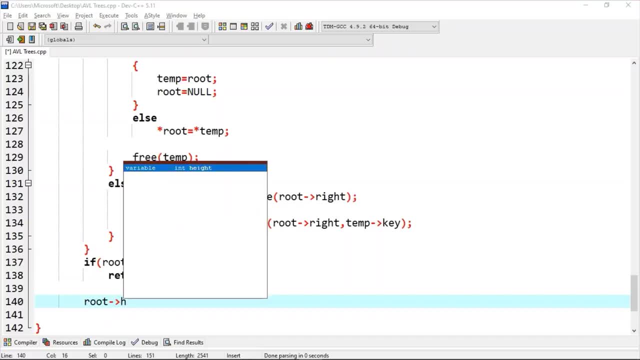 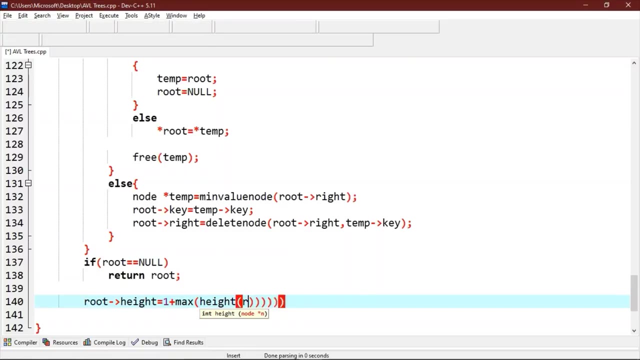 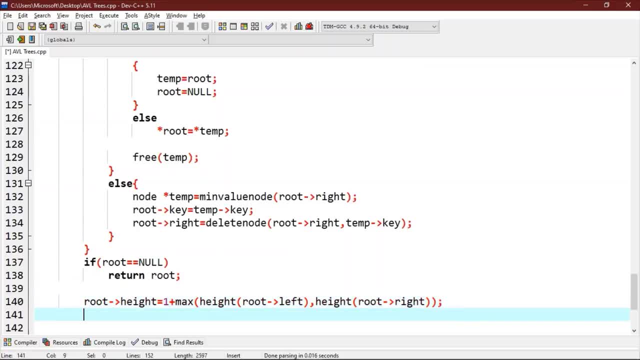 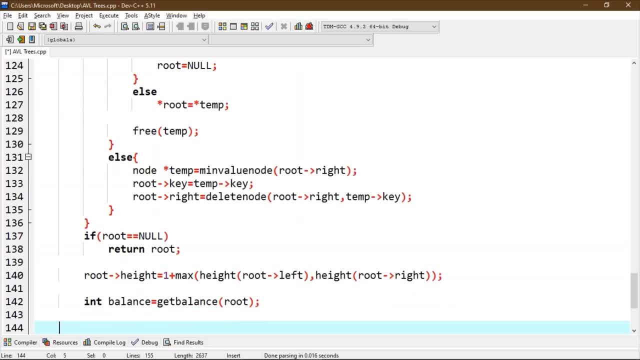 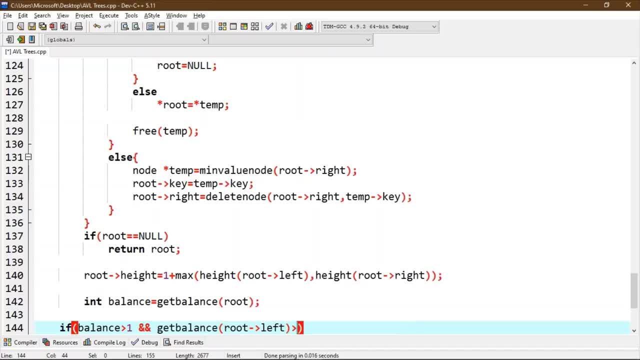 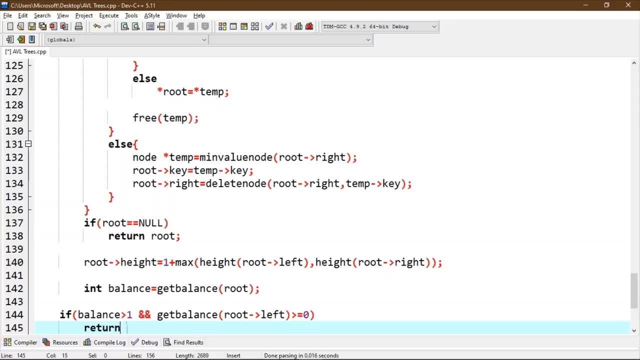 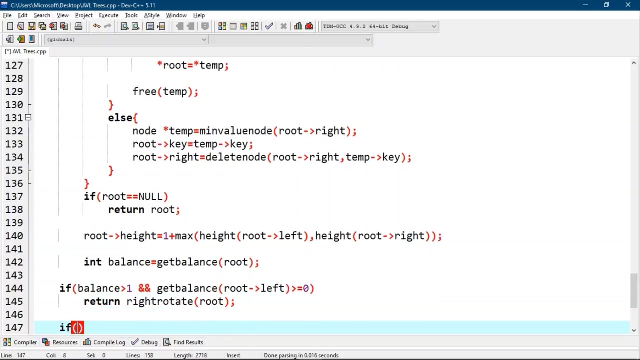 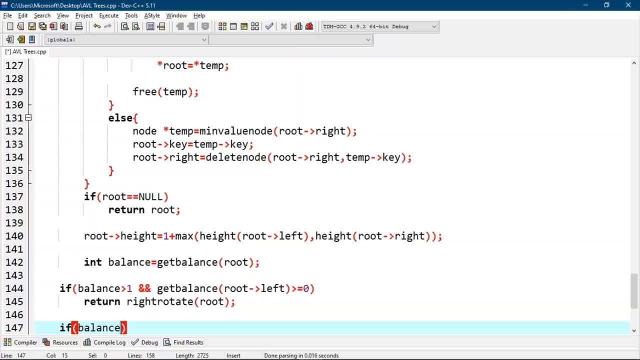 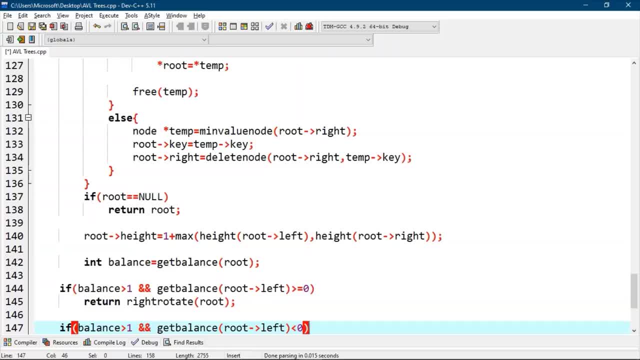 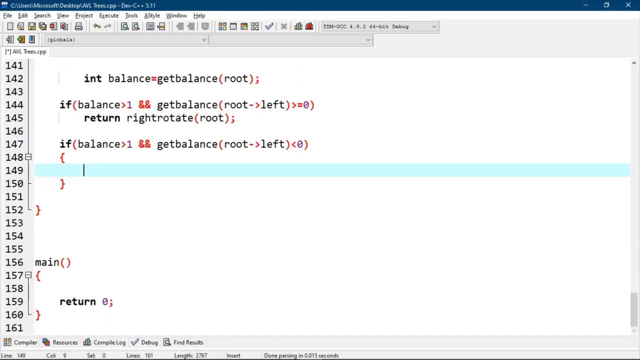 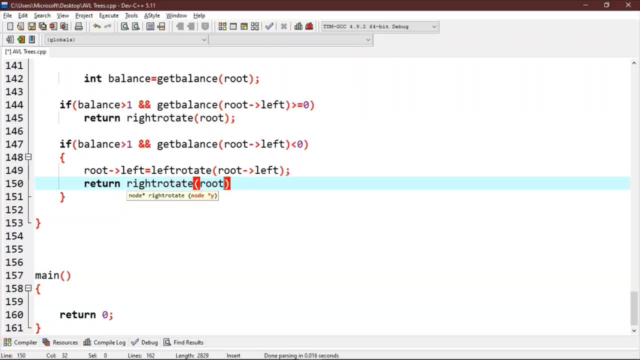 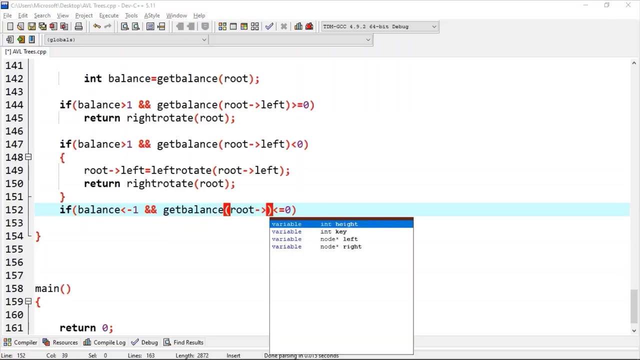 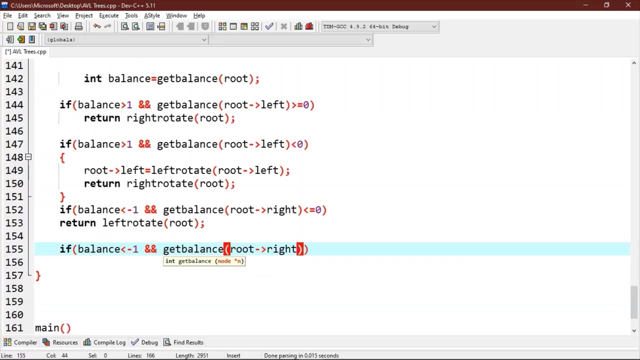 root. now let's write right right case. so if balance less than minus one and get balance is less than equals to zero, and then we will return left rotate. now we will write right left case. so if balance is less than minus one and get balance, of root right is greater than. 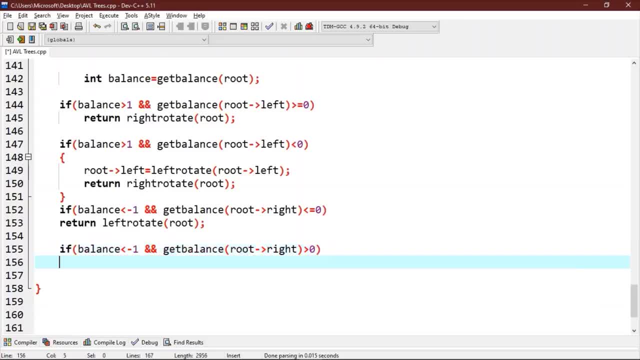 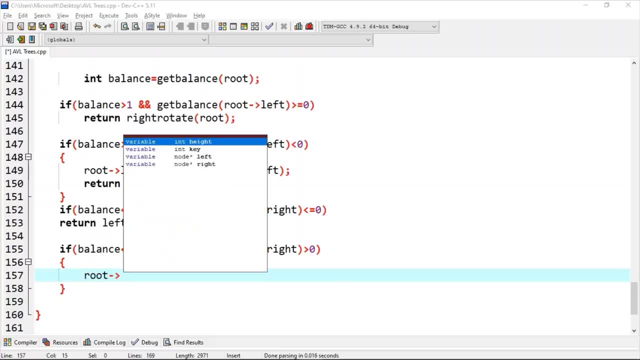 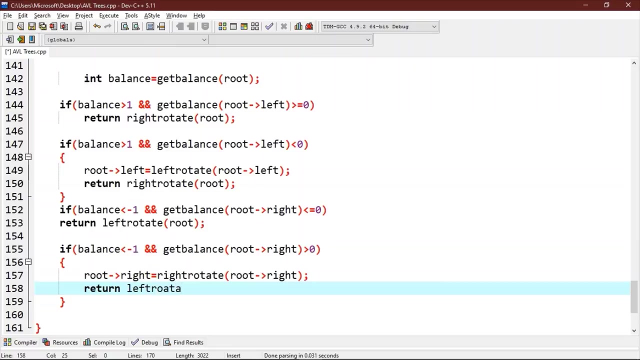 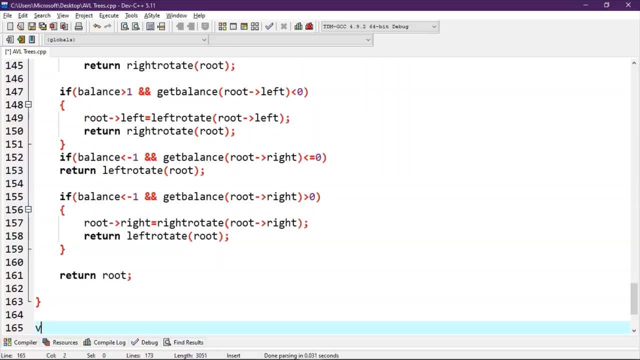 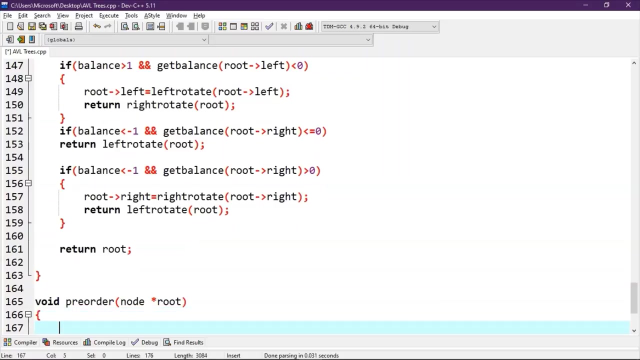 zero, then root right is equals to right rotate right now. we will return left rotate and we will return this root. now let's write a function to print pre-order traversal of this tree. so void pre-order node star root. pre-order traversal of this tree. so if 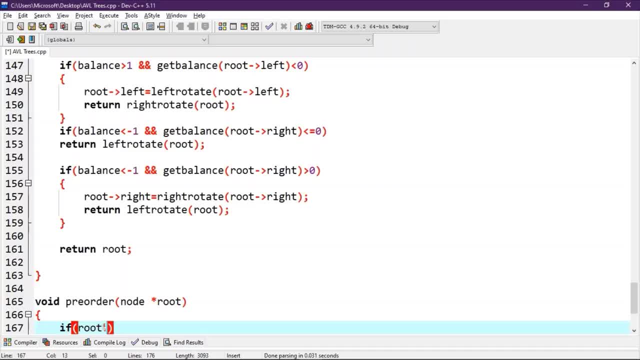 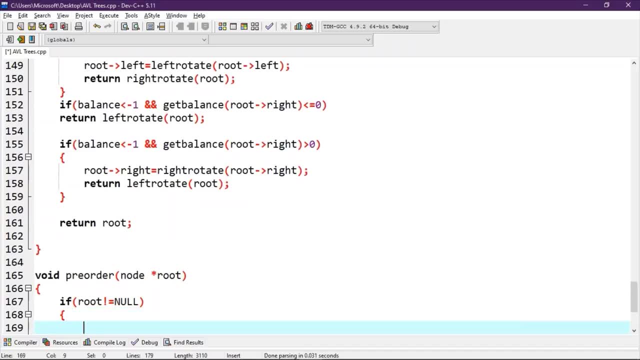 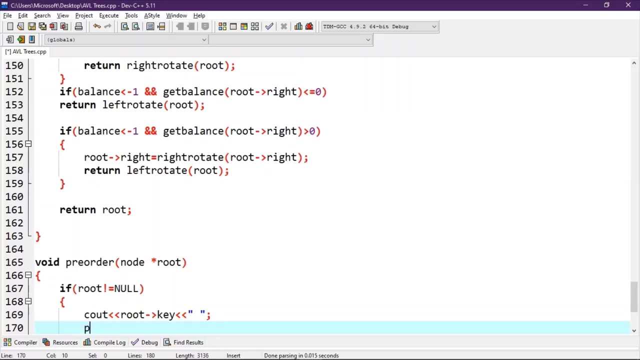 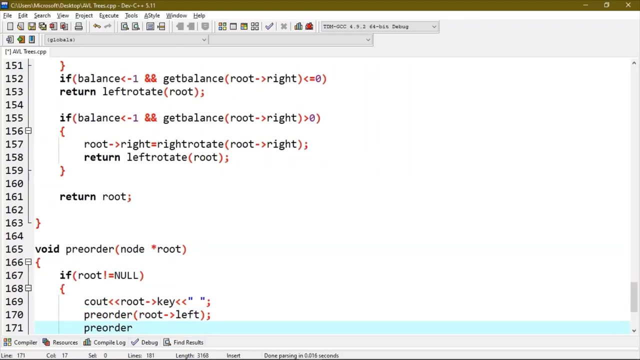 root not equals to null. and cout root e and cout root e and cout root e. enter pre-order root and end it with a sub pass and pre-order root. right now, let's write a code for the main block. let's write a code for the main block. 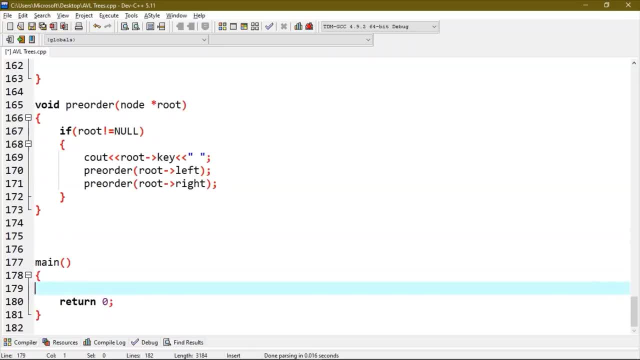 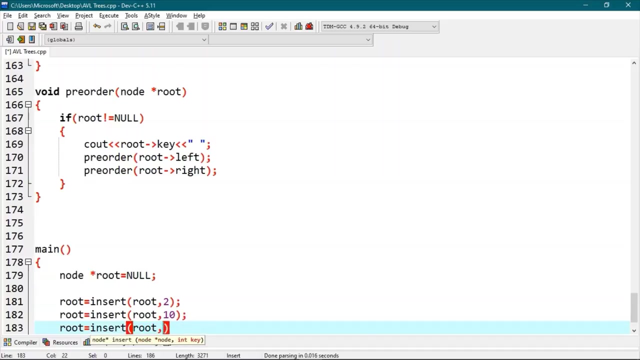 let's write a code for the main block. We will start with an empty tree, so node root is equals to null. now root is equals to insert root comma 2. root is equals to insert root comma 10. root is equals to insert root 10 comma 9. root is equals to insert root comma 7. root is equals to insert root comma 5. 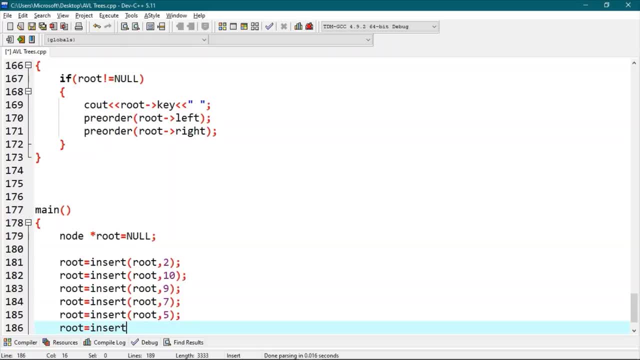 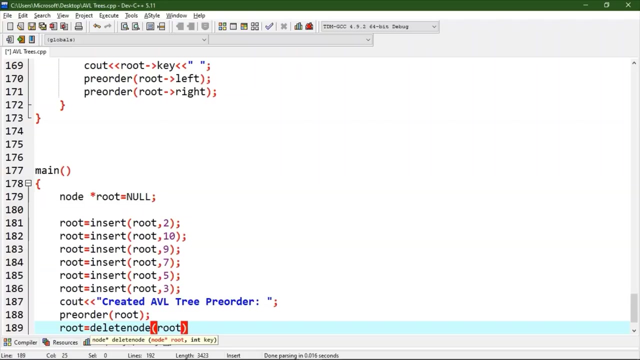 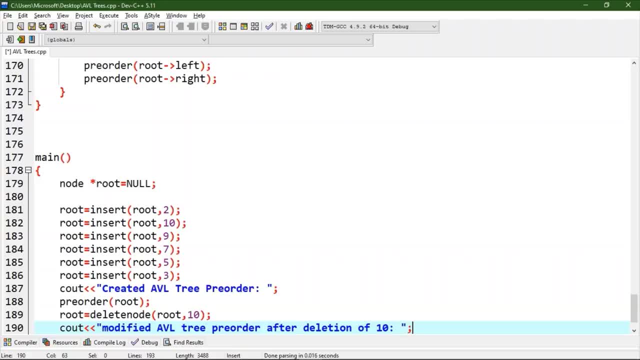 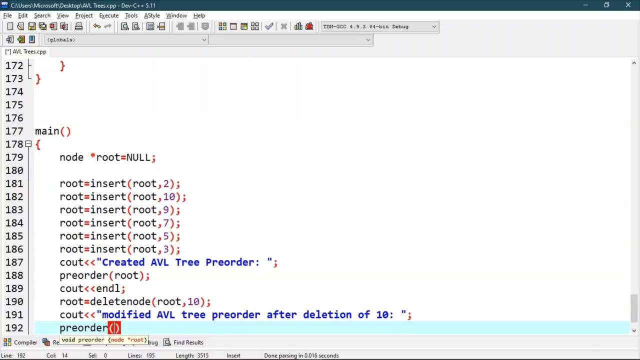 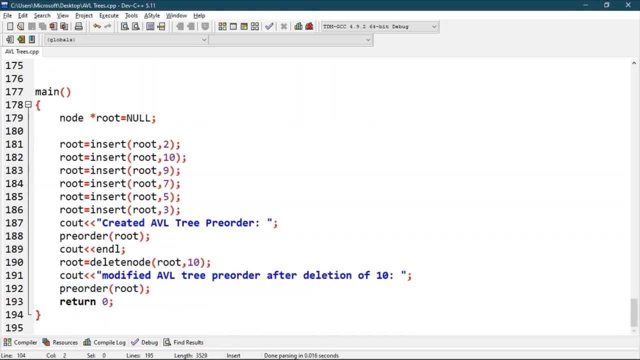 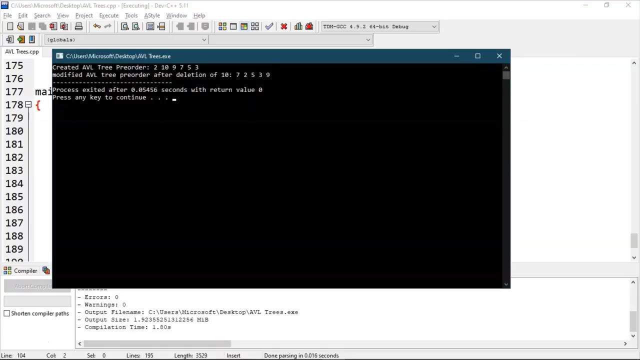 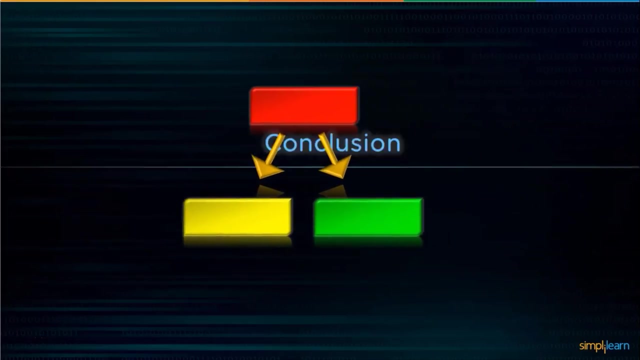 payout handle. pre-order route: delete. now let's execute this. as you can see, our deletion function is working perfectly. now let's get back to our slides. at last. let's sum up what we have learned from this session. first up, abl trees is our self-balancing. 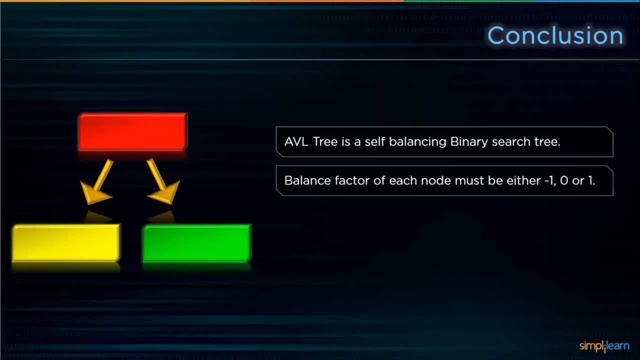 binary search tree. next, every node must have a balance factor of either minus one zero or one. next, after every rotation we must verify if each node is balanced or not. finally, avl trees offers fast insertion and deletion operations. and this was all for today's session. hope you guys found.